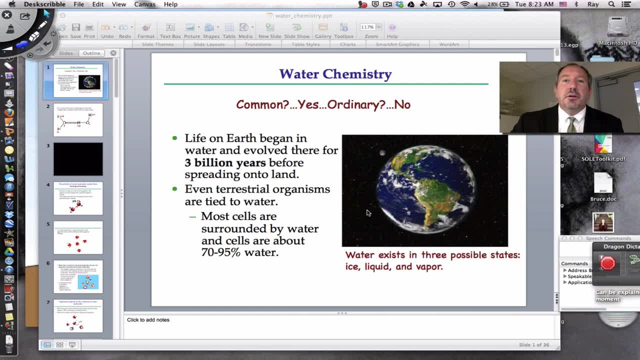 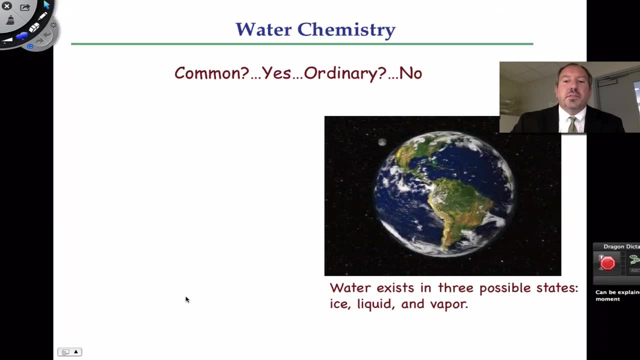 some of the characteristics of a water molecule, how they interact with one another, how they interact with other molecules and some of the emerging properties that are unique and somewhat extraordinary in water. And so let's jump right into that discussion. And so one of the things 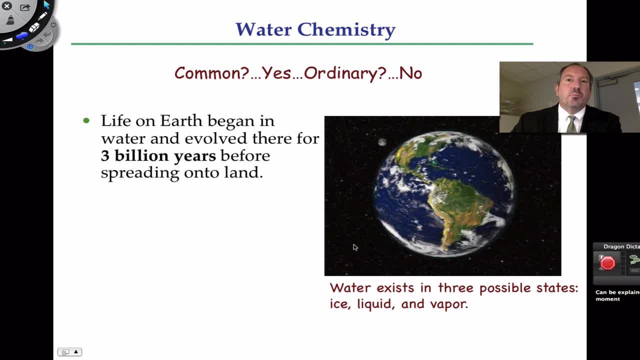 about water is that we could say that we believe. we're not 100% confident, but we believe that water perhaps began. life began in water about three and a half billion years ago and then spread onto the land. There's evidence that supports that, And our own cells are composed mainly of water, And 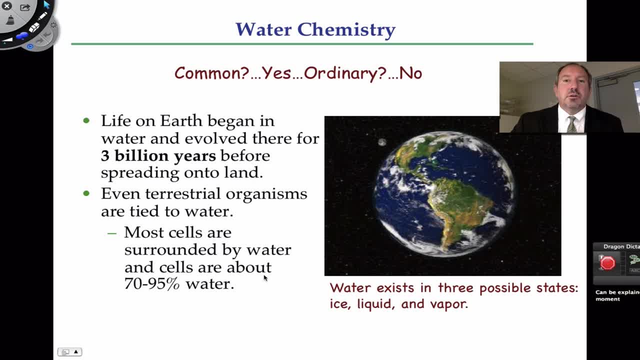 really, if you scale it up, organisms in general are mostly water, And so the study of biology is really the study of water, And so the study of biology is really the study of water, And so the study of water. And so the study of water is really the study of water, And so the study of water. 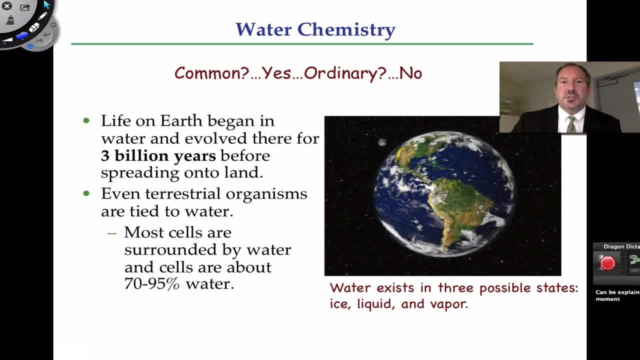 is really the study of water, And so the study of water is really the study of water. In other words, all of these chemicals like sugars and salts, and proteins and nucleic acids are dissolved in an aqueous solution, And so how water behaves is extremely relevant to our discussion of 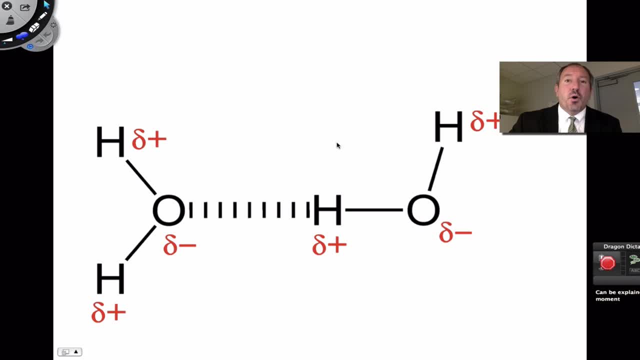 biology, And so all of that stems from the water molecule itself. So let's get into this. You might already know this, but just a review. Therefore, you might know that water is, and you also might know that there is a covalent bond between oxygen and 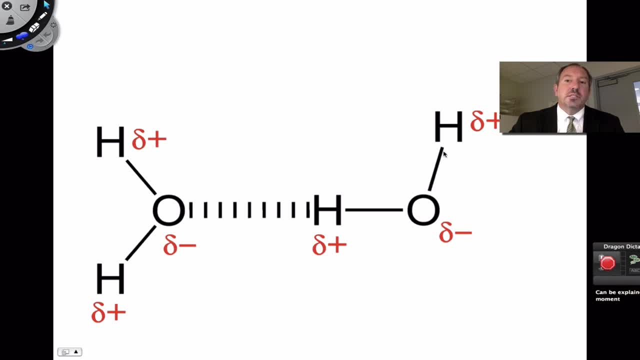 hydrogen right there. so there's two covalent bonds. but what's interesting about these covalent bonds is that they're polar. so this right here- see if I can label that- that right there is a polar covalent bond, so polar covalent. 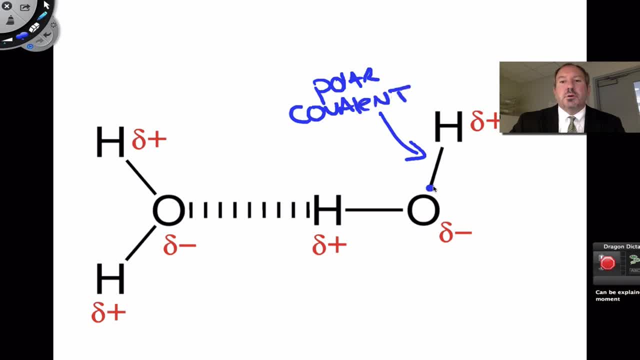 and that's really important, because if it's polar, that means that the electrons are hanging out a little bit more around the oxygen than the hydrogen, because, as you may recall, oxygen is more electronegative, so it's so it's like a tug-of-war and oxygen is winning it, not winning it so much that it could yank the. 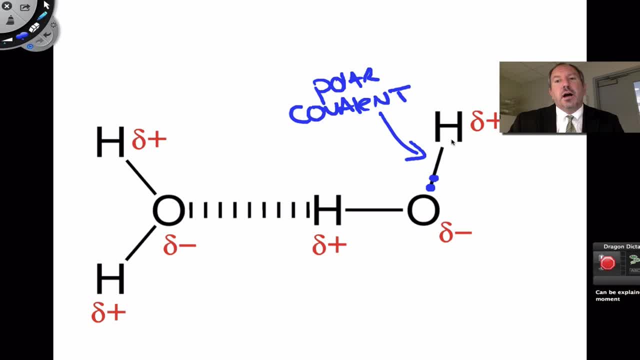 electron away from hydrogen, because that would therefore cause it to lose an electron, and then it would form an ion, a proton by itself, which is a hydrogen ion, and then this would have a negative charge. you so same things happening over here, and so do you notice how water? therefore, 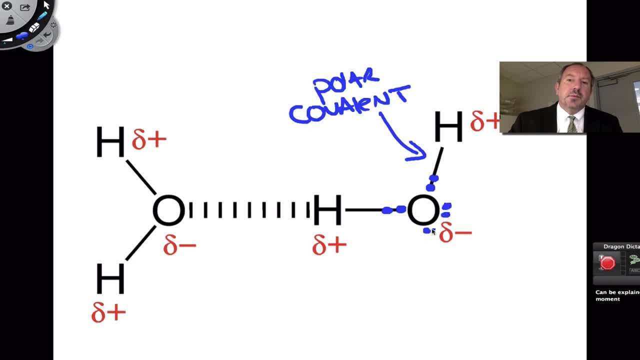 there's a lot of electrons, and I'm not even showing the free electrons over here. there's a partial negative charge on one side of of water and a partial positive charge on the hydrogen side. so, as a result, water is considered to be a polar molecule and through that polarity that OH bond. right there it's not the 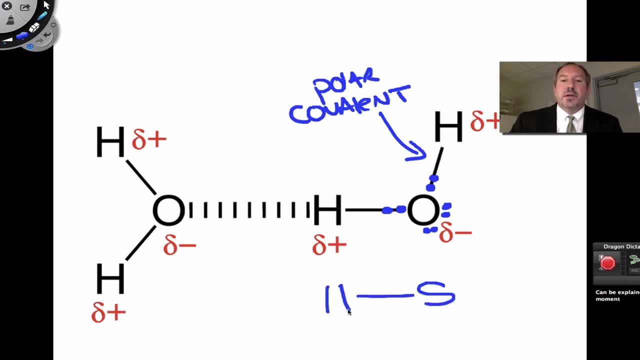 only polar bond. you can also have this as a polar covalent bond and this is a kind of a weaker polar covalent bond. so these are the ones that are very important but as a result of that OH being polar, it results in this being partially positive and this is partially 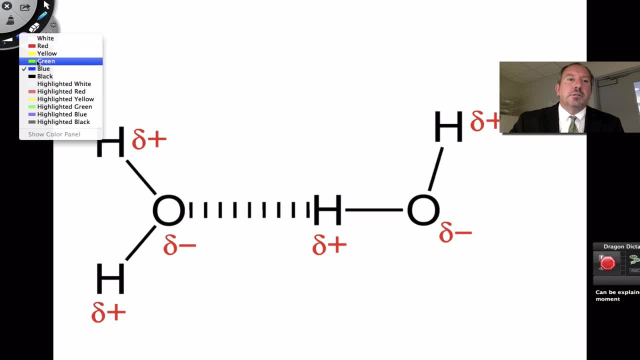 negative, and so this new type of bond emerges, and this is basically the. the central focus of all of the unique properties of water is based off of this intermolecular bond, which is called a hydrogen bond. Its an intermolecular bond from the superceurectalceeds to the nematode decade, episode from언ethe results this being partially positive, audiences partially negative. and so this new type of bond emerges, and this is basically the. the central focus of all of the unique properties содержes of water is based off of this. 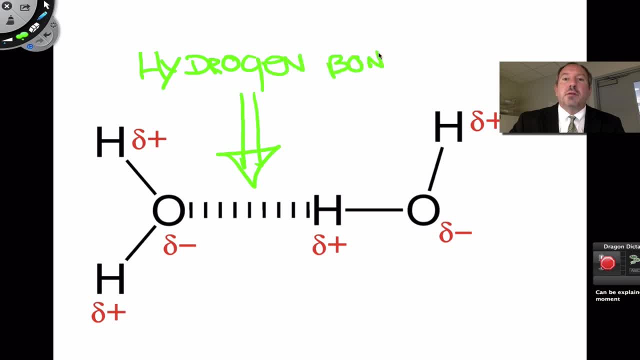 bond which is called a hydrogen bond. It's a bond between polar molecules And the reason that it's called hydrogen, I believe, is because it's always involving hydrogen. Do you see notice here like this? And it has to do with the electronegativities. Do you see how, as a result of the 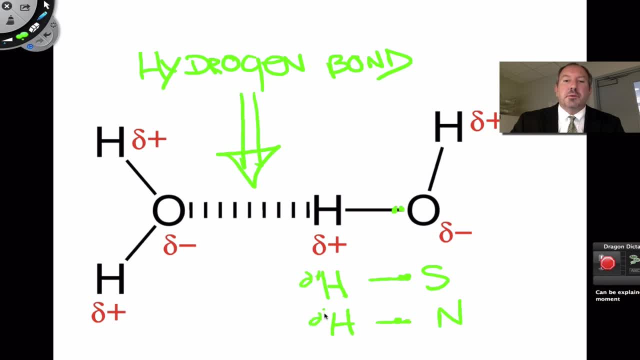 electronegativities. you get this partial positive over here. partial positive, partial positive. So it's called a hydrogen bond. If you're wondering, why isn't it called an oxygen bond? So these lines or little dots, represent a hydrogen bond and they're really weak. 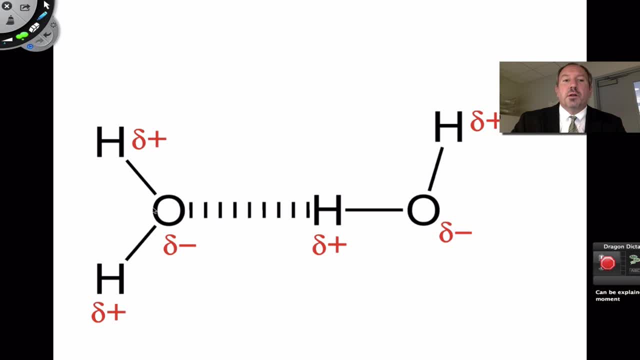 but they're strength in numbers, and it can cause one water molecule to stick to another, And so this is called cohesion, if you recall that somewhere in your chemistry past. if not, welcome. Cohesion is hydrogen bonding between the same molecule, in this case water, to water. 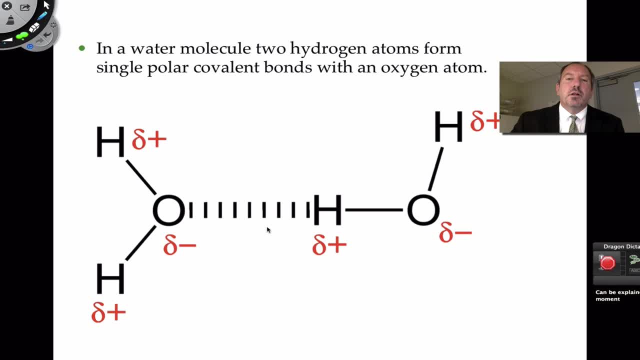 So there's cohesion between water molecules, And so water molecules have these two hydrogens that are partially positive, and that there is single polar covalent bonds with the oxygen, And so, as a result of that, you get some interesting things happening, Because if you have, 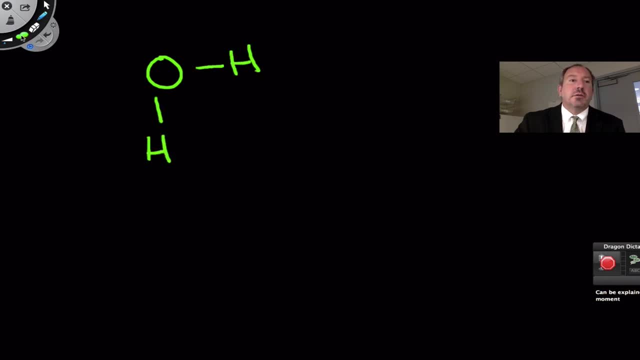 one water like this and it's close enough to another. you can have things like this. you can have hydrogen bonds forming like this between another water molecule like this, And so hydrogen bond and this is cohesion between the water molecules, because this is slightly positive. 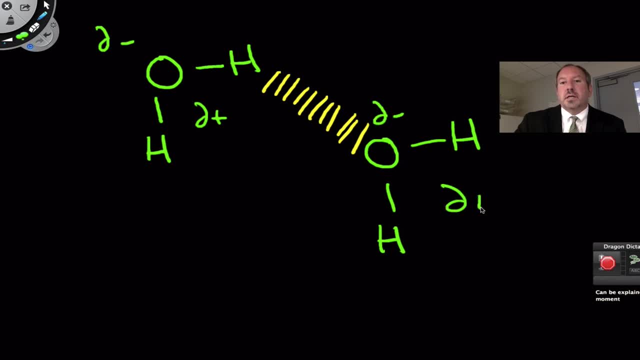 over here. slightly negative, slightly negative, slightly positive. So this is a hydrogen bond, And are you ready for this? Hydrogen bonds are pretty much the reason for all of the unique properties of water that we're about to discuss in this video. So there you have it. So the polarity. 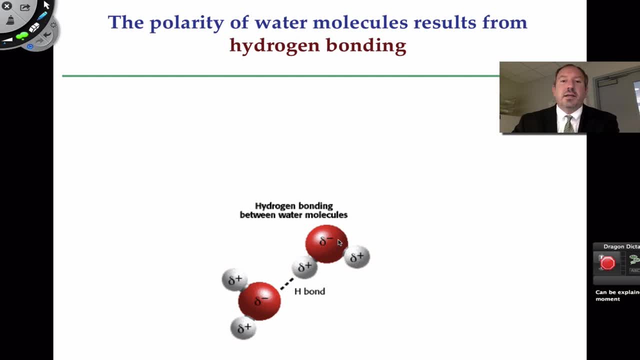 of water results from hydrogen bonding, meaning as a result of the polar bond between the oxygen and hydrogen, hydrogen bonds will form, And so this dotted line represents the hydrogen bond, and so they stick to one another. So water sticks to itself, And so that's pretty interesting, As you can see here in this picture. 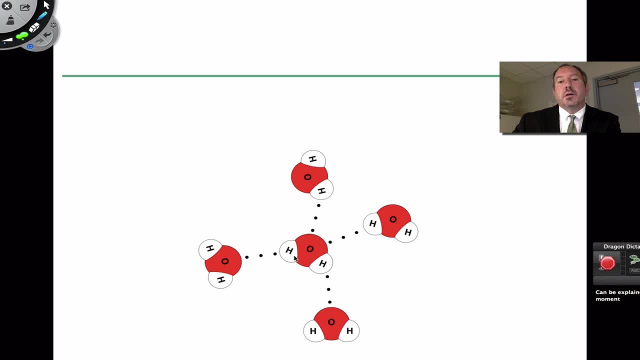 water forms four possible hydrogen bonds with other water molecules, and let me just add this first one, and about the life to it will be none concepted or possible. as you can see here in this picture. water forms four possible hydrogen bonds with other water molecules. and let me ihr. 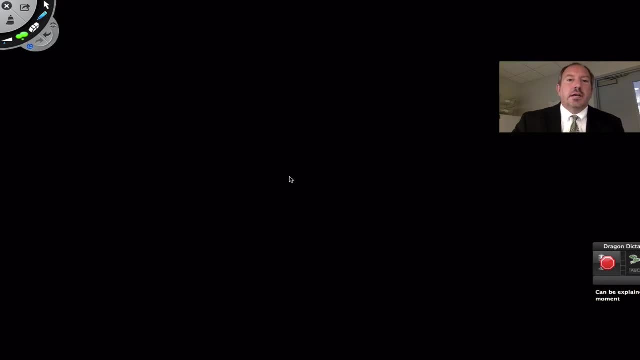 me go back to this dark screen so I can illustrate that. If you had a water molecule like this, sort of v-shaped like that- and this is partially positive right here, this is partially negative over on this side. So I'm going to draw. 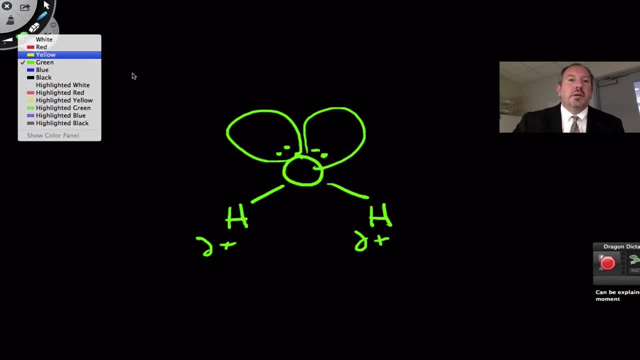 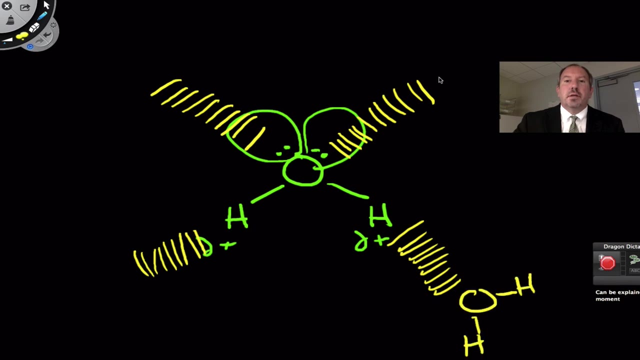 on the free electrons right here. So what could happen is you could hydrogen bond here and here and here and also here. It can form four hydrogen bonds. So there's a water over here would be a water like that, and this would be a water like this. 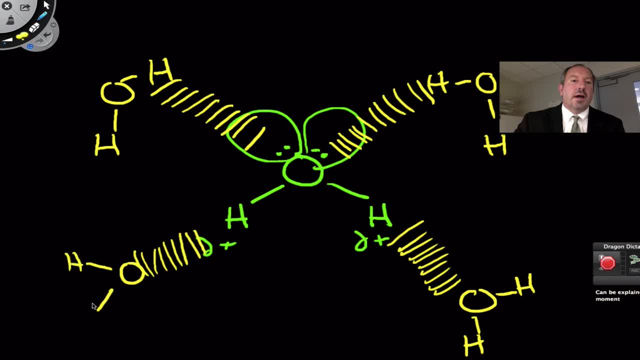 and this would be a water like that. And so you're like, wow, I didn't realize. water can form four hydrogen bonds with other water molecules. Well, it does and it doesn't. It all depends on how fast the molecules are moving. and so this is a. 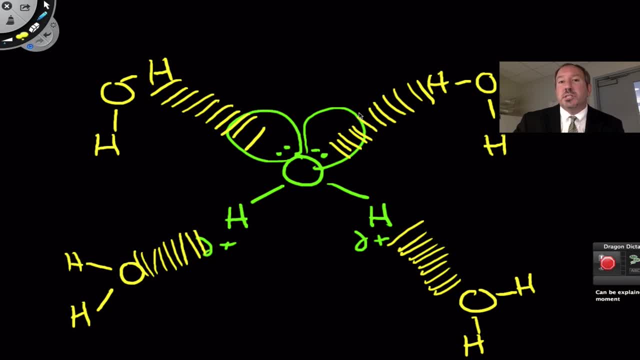 measure of the kinetic energy, the speed at which the molecules are moving. It's sort of as if you were holding hands with friends. If I had you hold hands with your friends and stand still, it's like, yes, I can do this, But 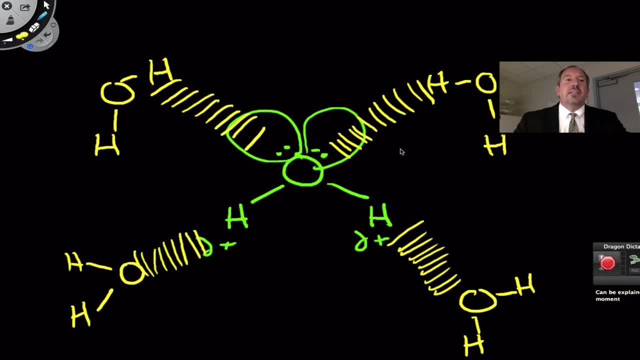 if I asked you to move around, you could still sort of maintain that. but if I had you run around, what would happen is you'd be throwing your friends all over the place, and so 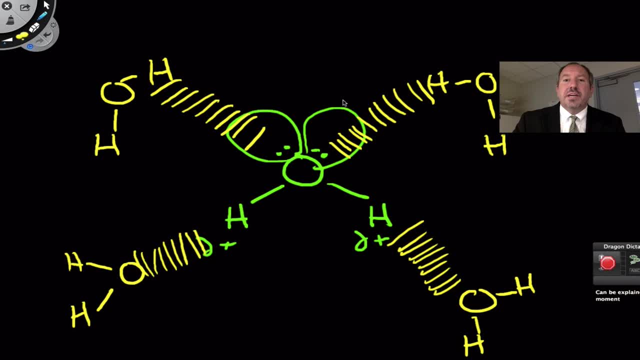 When you increase temperature, it very easily breaks these hydrogen bonds and therefore it forms less of them, And so the water molecules can get very close together. But this would be a picture like an ice, And I'll come back to this point because it's rather significant. 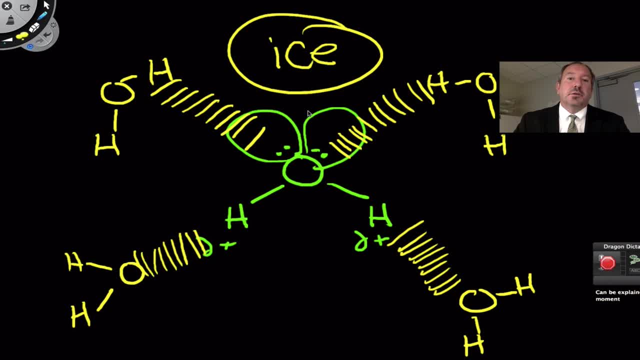 So when the molecules are moving very slowly- in the case of cold like 0 degrees Celsius- it can form all four of its hydrogen bonds. And the reason that that's significant- I'll foreshadow it- is that there's a lot of space in between the molecules. 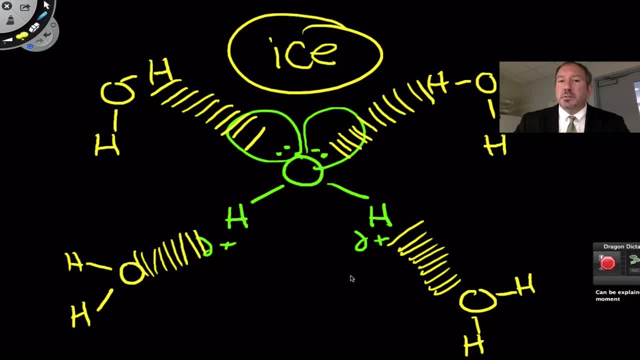 And so, therefore, there's less water molecules in a given area, therefore less dense than liquid water, which would be moving more quickly, And so there'd be more water molecules in liquid water in the same area than there would in ice. Less water molecules, therefore less dense, in the same area. 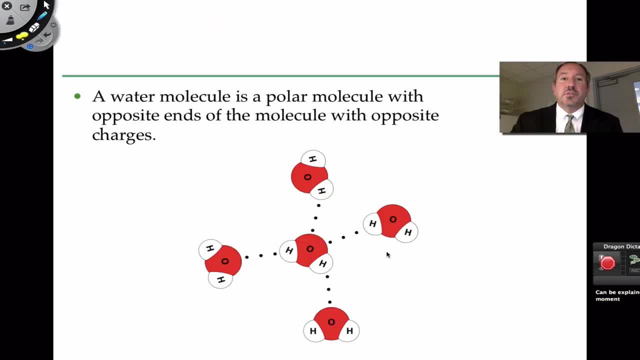 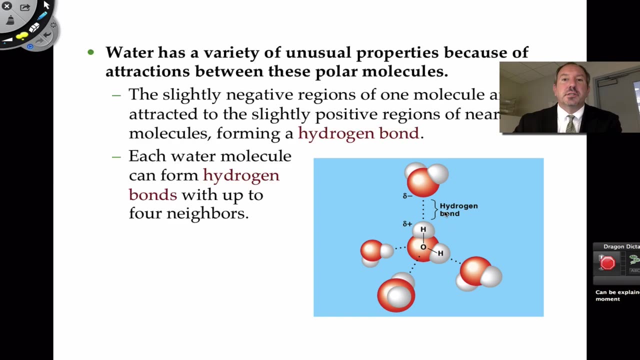 So that's rather significant because ice floats Because it's less dense, less water molecules, And so this would be like ice. So water is a polar molecule and it hydrogen bonds with itself and that's an example of cohesion. So there's another picture, a lot of pictures. 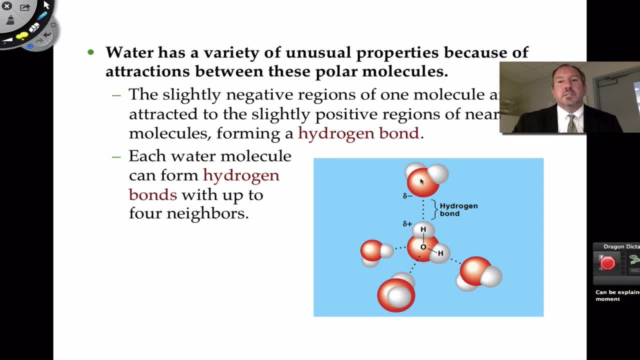 If you want more examples, the internet is very good with this. And so these hydrogen bonds. I'm labeling hydrogen bonds red here, because all of these unusual properties about water are really the result Of hydrogen bonding between water molecules, because there's an interesting things that emerge as a result of it. 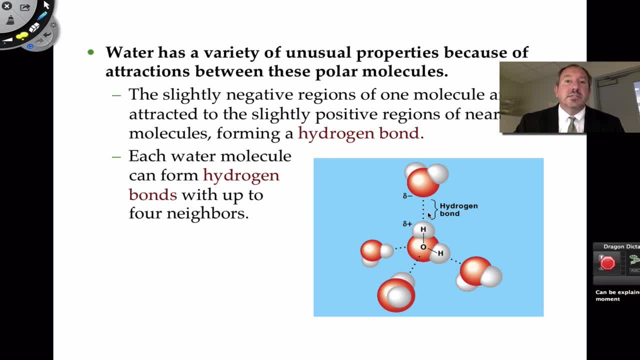 So, now that we've established that a hydrogen bond is an intermolecular means between molecules, and it's weak, but there's strength Because if you have a lot of water molecules, there's a lot of hydrogen bonds, And so, though the bond itself is weak, there's strength because there's so many hydrogen bonds. 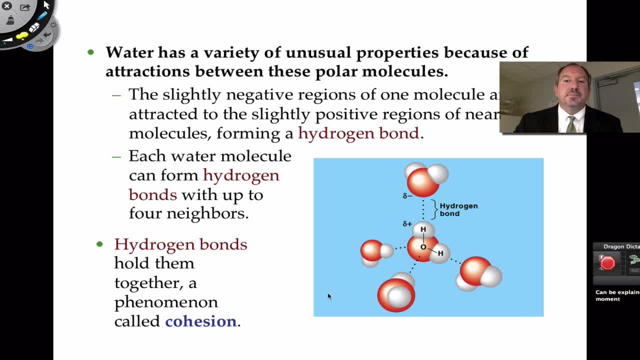 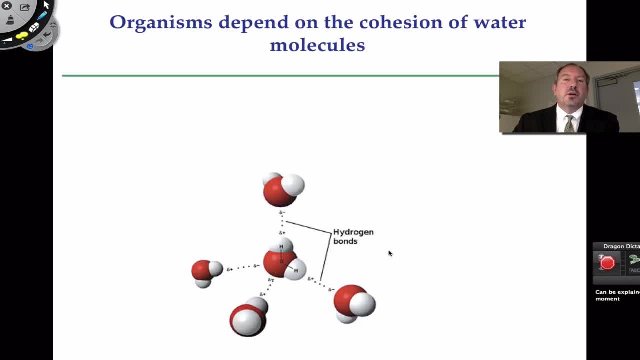 So that is important. I threw out this term, cohesion. This is a great picture of cohesion, In other words, water-hydrogen bonding with itself, And so organisms depend on the cohesion of water. You're like well, really. 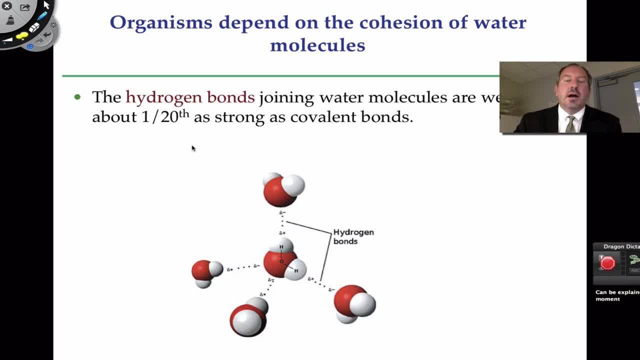 Yeah, and I mentioned the strength of water. I'm sorry, the strength of a hydrogen bond is only 1, 20th that of covalent And you're like, ah, it's weak, But again, there's many of them. 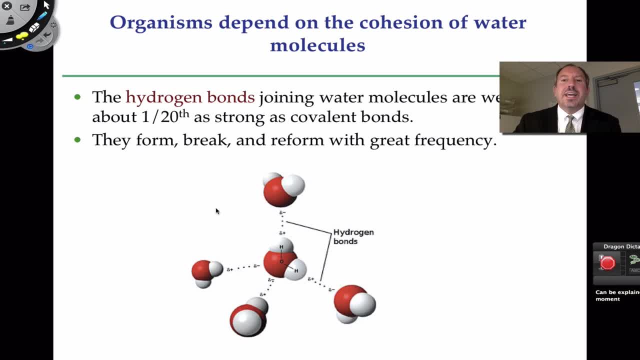 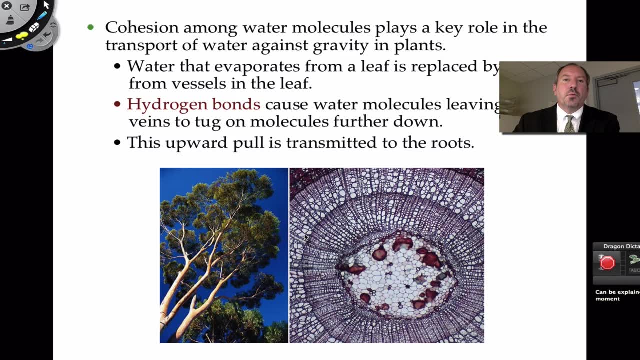 So it culminates into strength, And so They break and form with great frequency. They're forming, they're not forming, they're forming, they're not forming. And so when I say that life is dependent on this is one of the great examples of cohesion is the fact that water can move up a tree. 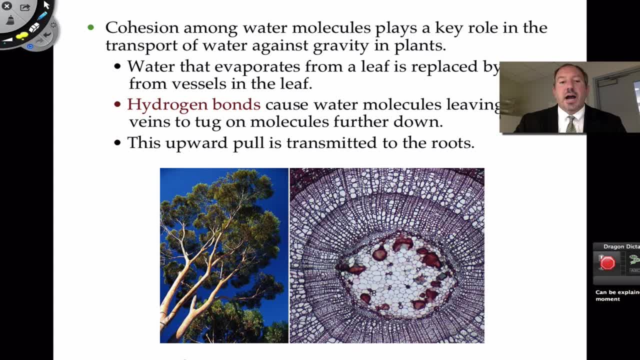 Now I don't know if you've given this thought before, but how can water, literally when it rains and it goes into the soil, how can it go up hundreds of feet into a tree? I mean, it's defying gravity. 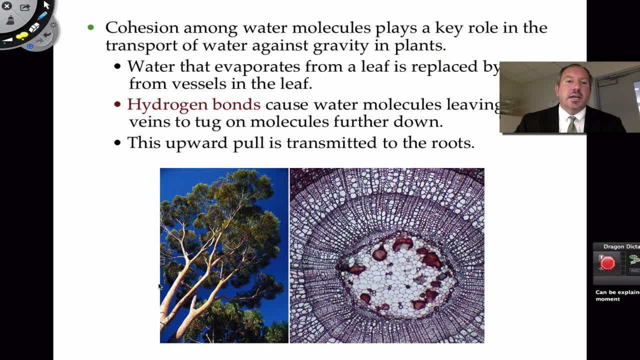 You're like I don't know, I'm not really. I don't know if you've considered it. Well, if you were to take a cross section of the stem like this and take a look at this under the microscope, what you'll find is these little circles are the cells. 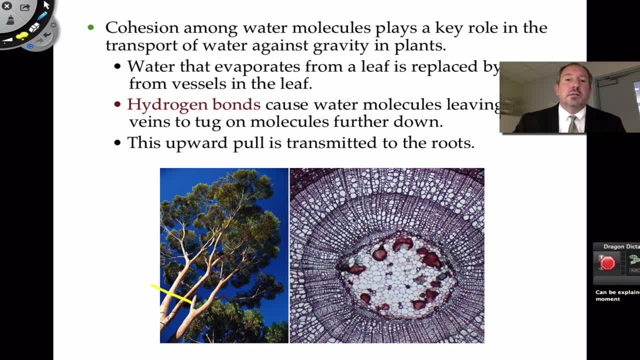 And it's a special tissue called vascular tissue And in particular it's called xylem. And xylem are like straws. They're very elongated, cylinder-like cells that are hollow. They have a thick cell wall which gives them strength. 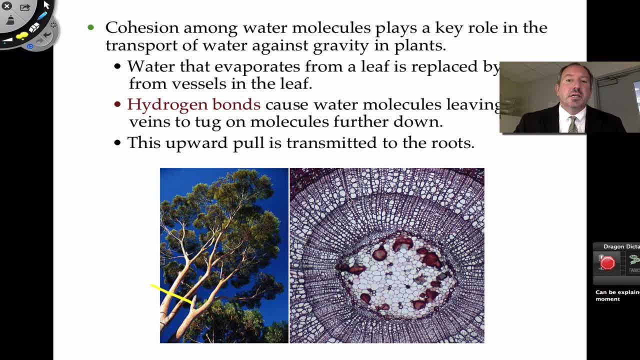 And it makes wood very strong, And wood is It's vascular tissue, And so water travels up these straws, So it's like looking down at a box of straws right there. So how is it that water can move up? Well, if all the water molecules are connected together like this, they're all connected together through cohesion. what happens is at the very top in the leaves when water evaporates, in other words, it transpires from the leaf. since all the water molecules are stuck together, it's simply it's not going to move up. 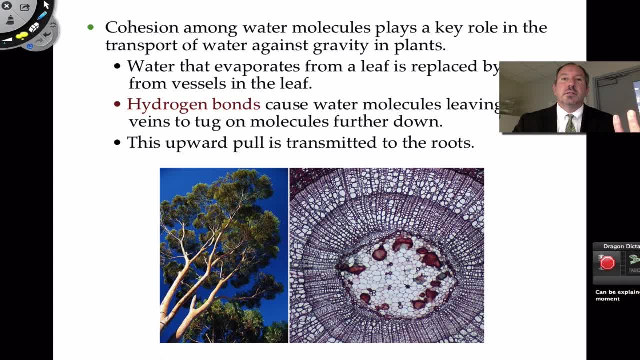 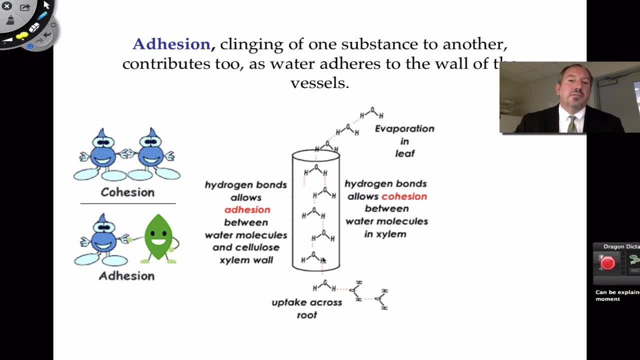 And so the truth is, the fact that water is sticking to itself is only part of the answer. So that's cohesion, And remember, the pull is caused by the evaporation of water from the leaf- But there's also adhesion. Adhesion is where water molecules can stick to a different polar molecule, like, in this case, the cell wall. 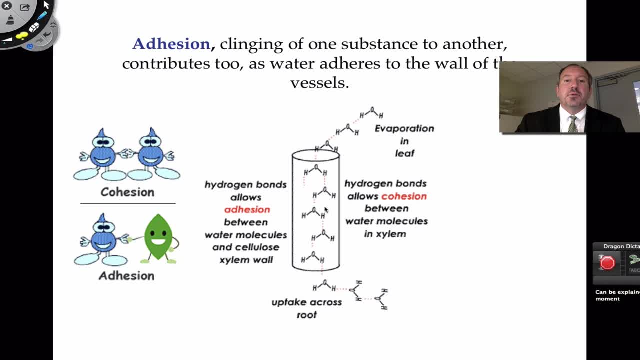 So adhesion, in other words sticking to something. so it's like climbing the ladder and it's all stuck together. So cohesion and adhesion is why water moves up a tree. Together, these two phenomena make up what's known as capillary action. 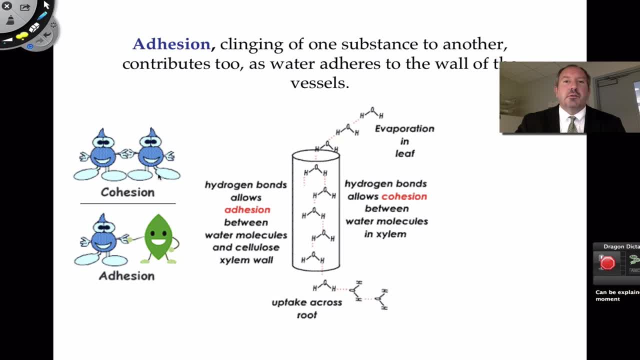 Capillary action, how water moves up, And so I found this diagram to be kind of humorous. Cohesion is water to water, and adhesion is water to something else, in this case like a leaf, Sometimes adhesive tape. sometimes we know it by the brand scotch tape. 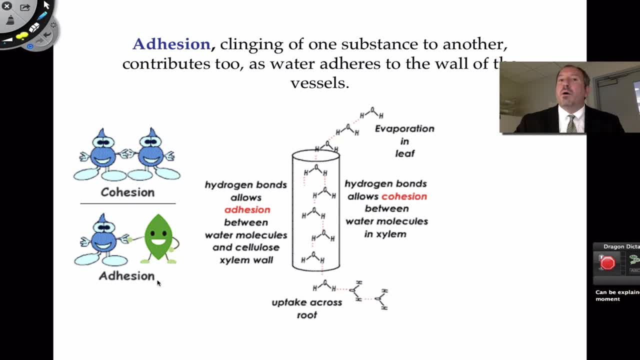 But adhesive tape can stick paper to a wall like that, So two different things sticking together like water to something else, So adhesion. So let me just come over here and show you what I'm talking about in terms of like a little animation. 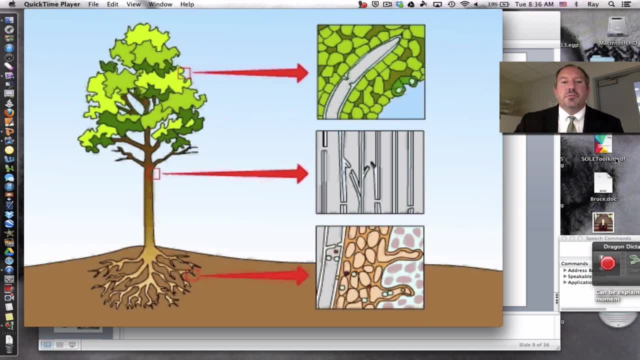 Do you see here, like in this diagram, water enters into the root, And as it enters into the root, it diffuses. It diffuses across the root into the vascular tissue. The vascular tissue is shown here in gray, And what's interesting about that is that it's the hydrogen bonds that are allowing the water molecules to stick together through cohesion. 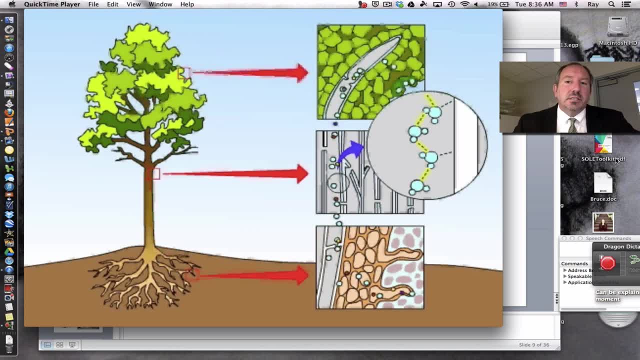 but they're also sticking to the cell wall, which is adhesion. So there's the hydrogen bonds, cohesion, And then when they stick to the cell wall, it's considered to be adhesion. And so you can see like, all right, if water is all stuck like that, then it should be able to. 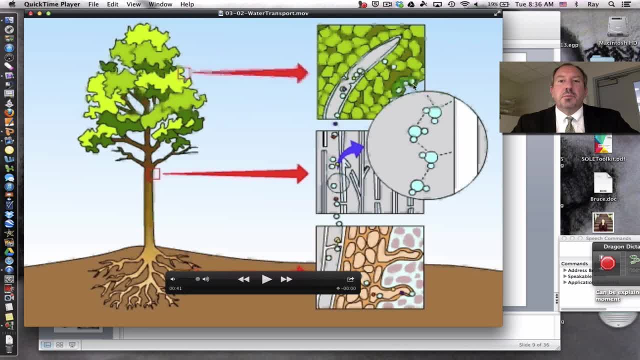 when it evaporates through these pores in the leaf called stomata, it should be able to make its way all the way to the top, And so it's a pulling action. Pretty, pretty cool, I think, And so let's go back over here if we can. 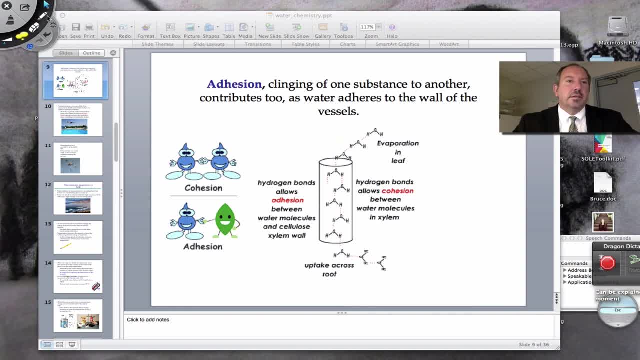 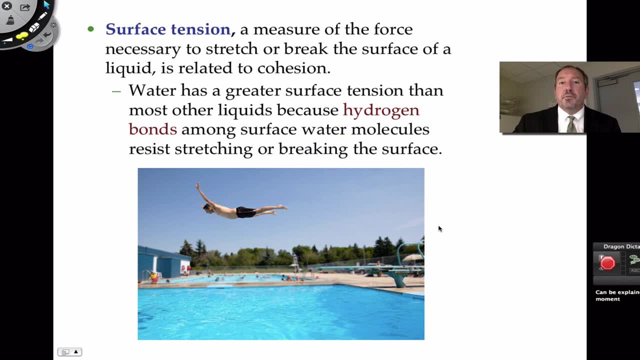 There's always a question of whether or not we can, And so, yes, we can do it, And so another interesting property of water- you're probably familiar with some of these- is surface tension. Now, I mentioned that. you know, water is such a soft, fluffy molecule. 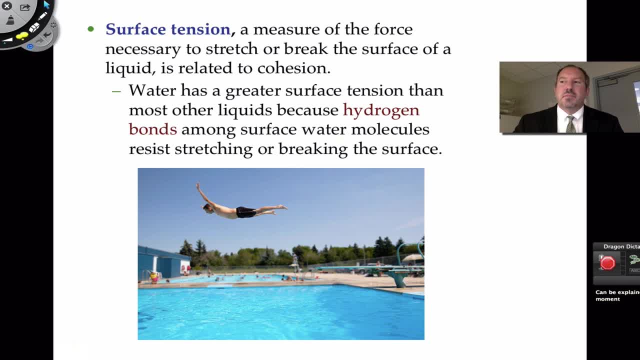 We like to get to swim in it. It seems rather, you know, benign in terms. how can it hurt us? But if you would never want to do this right, you would never come off of a diving board and go flat like that under the water. 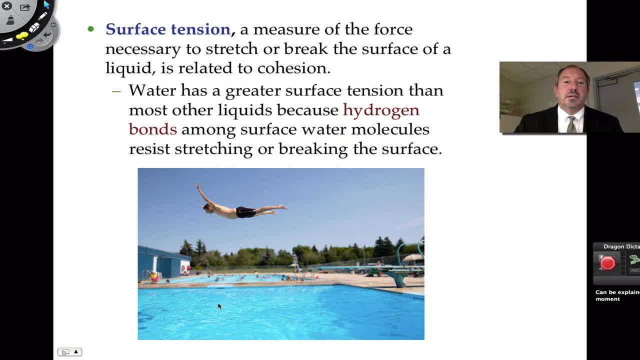 That would really, that would be really be smart, That would hurt. You'd smack that water and you're like: well, what is it about water That causes a belly flop? And you're like, well, I think there's some kind of surface tension that occurs in water. 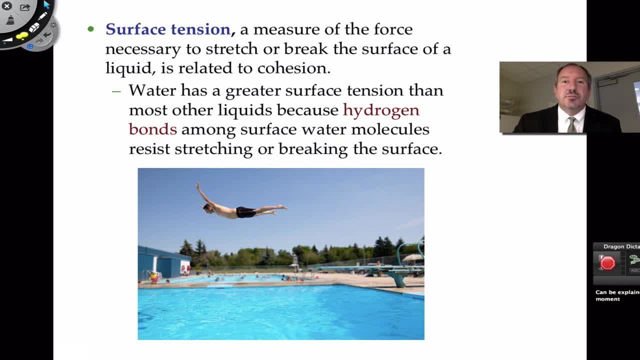 I'm not really sure. Well, it's the result. Again, the answer to all of these properties like surface tension is hydrogen bonding, And so difficult to draw this, but I'll try. Like if you had one water molecule like this flat, and then it was hydrogen bonding with another one like this you would have. 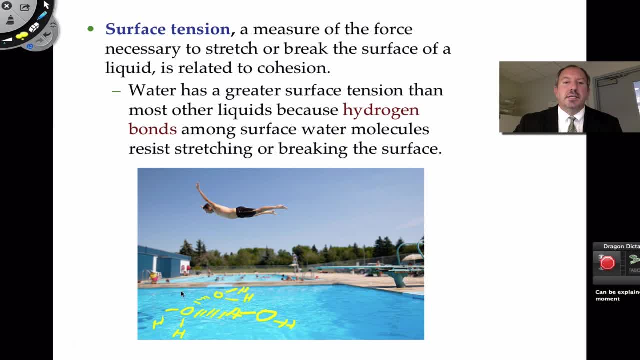 What amounts to as sort of like a spider web, an invisible spider web. Or if you've ever been to a concert and somebody is on the stage and they're like going off, and then they decide to jump out into the crowd And if the crowd were to hold its arms out, they might be able to catch the musician in their arms. 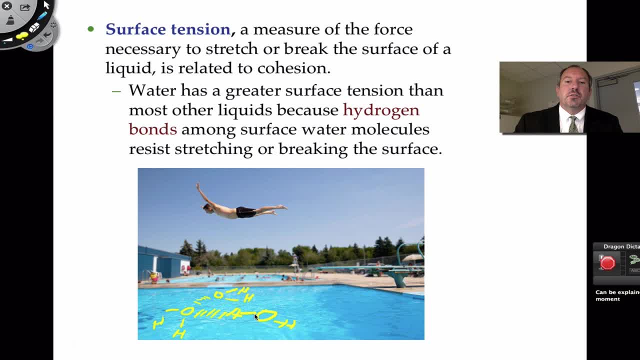 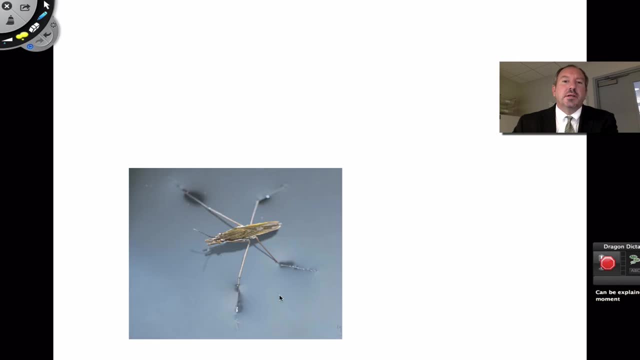 And so these hydrogen bonds that form on the on the surface of the water, are rather formidable, And so this, this is the result of surface tension, And so that's that's fairly interesting. And so some organisms could really benefit from this, Like, for example, some organisms like insects can walk on water. 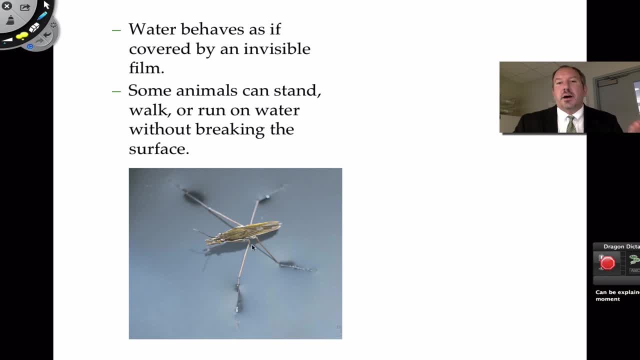 And what's interesting is, you know, if you have a lot of weight, obviously you're going to be able to break that surface tension. But the thing is some of these organisms have flat feet or these pads sort of like walking on snow. 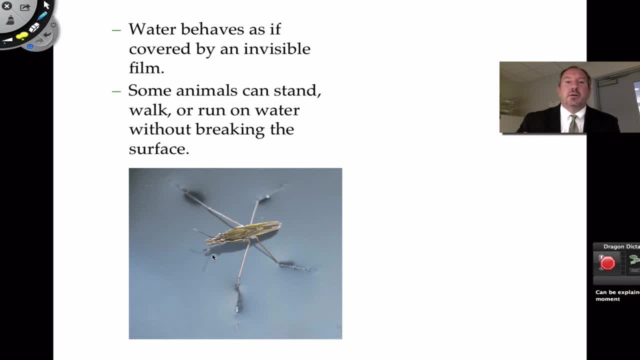 Like a polar bear has a very large foot, or it's like a snowshoe has, is sort of like a walking on tennis rackets, where it disperses the weight And so it allows you to stay up, And so surface tension is rather important. 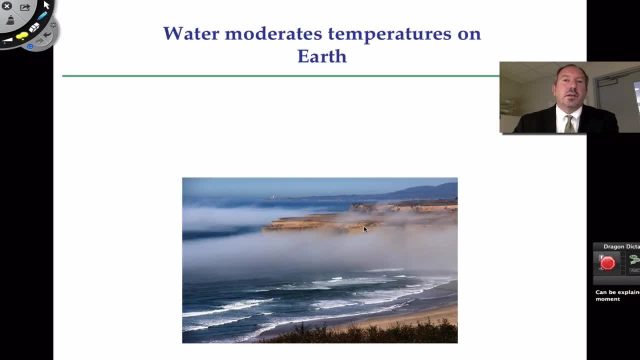 It's pretty interesting, And so one another interesting property of water- And this one is slightly complex And so I'll be returning to it a couple of times- Is that water can moderate the temperature Of the earth, And so what's fascinating about this is that you know, if you, if you live along the coast of California like this, you'll know that the temperature is always kind of moderate, meaning that it doesn't get very, very, very hot and it doesn't really get very, very cold. 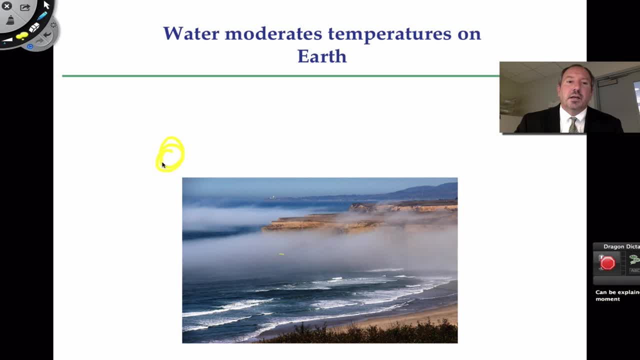 And it has to do with water. now, when the sun is shining like this, it's coming in, the heat's coming in and it's hitting the water, and the water, that heat, speeds up the molecule And it's it's breaking these hydrogens. And it's. it's breaking these hydrogen bonds, but it's absorbing the heat, absorbing the heat and then in the evening, new hydrogen bonds when it's cooler form and that releases heat, and so that it doesn't get very cold at night, doesn't get very hot during the day. 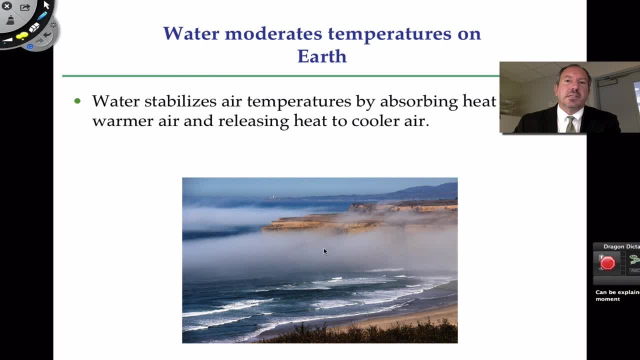 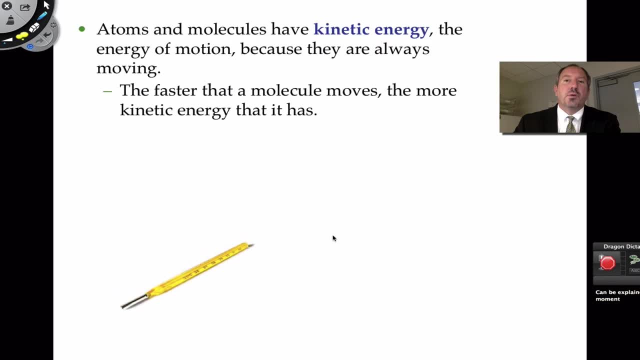 And I'll come back to that- And so it helps to stabilize air temperature by absorbing heat and releasing heat, and it has to do with hydrogen bonds, And so one of the things that that is important to consider is The fact that I alluded to this foreshadowed. it is that the molecules move, and that's when motion is a form of kinetic energy. 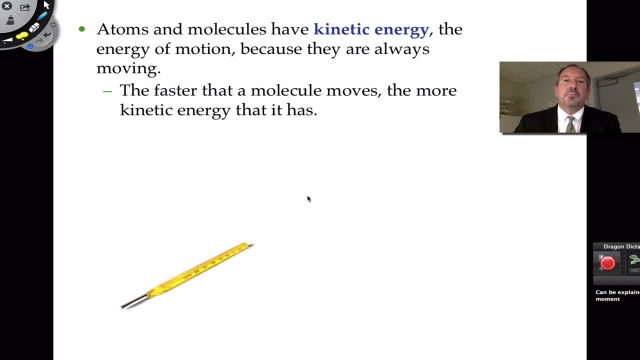 And so when the molecules are moving around, a measure of that is temperature. It's a measure of the intensity of heat due to the average kinetic energy of the molecule, And so we can measure that kinetic energy with a thermometer, And so obviously you're familiar with this. 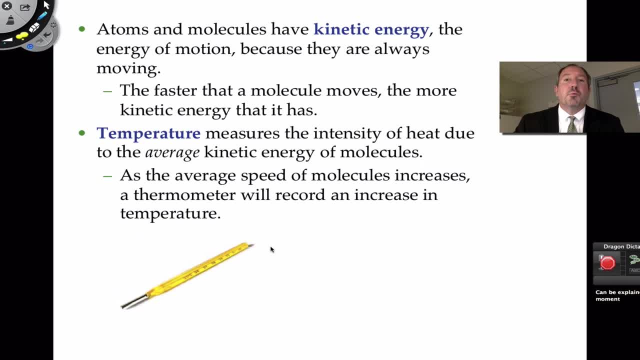 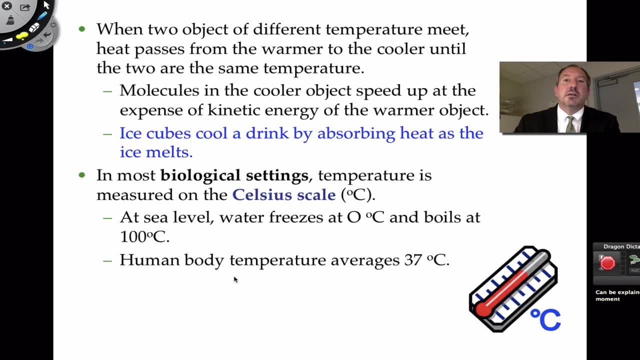 And so if the molecules are moving very quickly, it's a warmer temperature. If they're moving very quickly, Very slowly, It's a warmer temperature, And so one of the things that we like to consider in biology is that we like to use the temperature scale of Celsius. 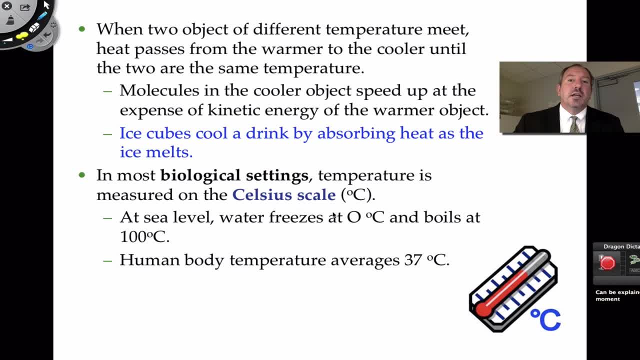 It's really within the range of biological organisms, That is, it's the CSI unit, the metric unit for temperature. You can also use Kelvin for this, But again, Celsius is a little bit more appropriate for biological purposes. So you may know that water freezes at zero. 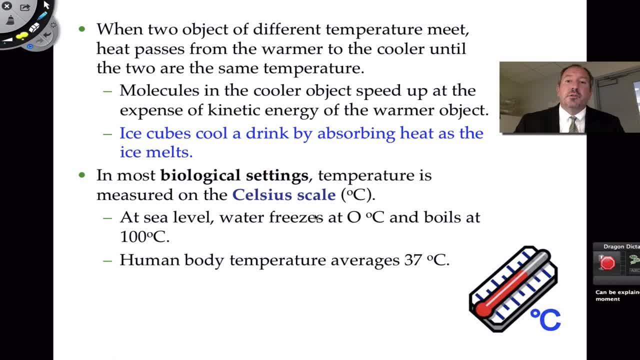 And it boils at one hundred. So those are two numbers that are significant to us. We also want to know that our body temperature is thirty-seven degrees And that average room temperature is about twenty-five. These are the numbers that we like to consider. 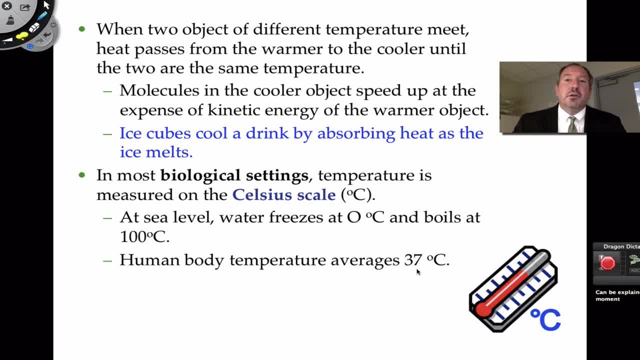 And again, this is kind of a trivial point, but it's kind of cool. So when two objects of different temperatures meet, did you know that the warmer one passes the heat to the colder one, And so molecules are moving, So we can measure temperature. 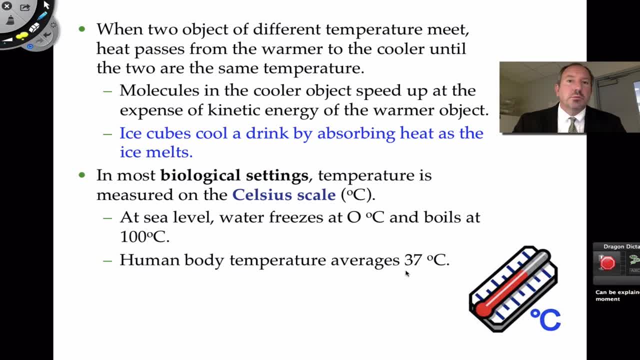 And so we're going to take the temperature how the temperature goes. it's not going to be the same as the previous one, But we're going to take the temperature how the temperature goes. We're going to take the temperature how the temperature goes. 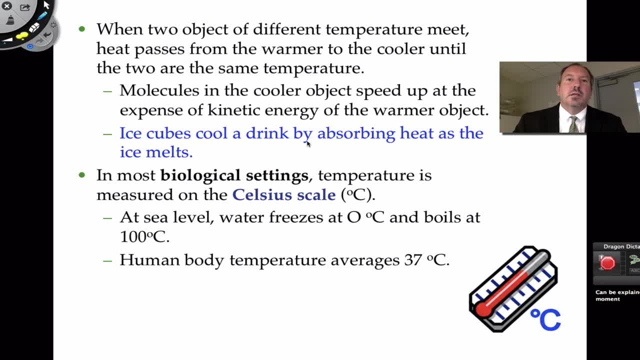 If we take the temperature of the water, then we get that temperature. These are the numbers that we like to consider And again, this is kind of a trivial point, but it's kind of cool. So when two objects of different temperatures meet, did you know that the warmer one passes the heat to the colder? 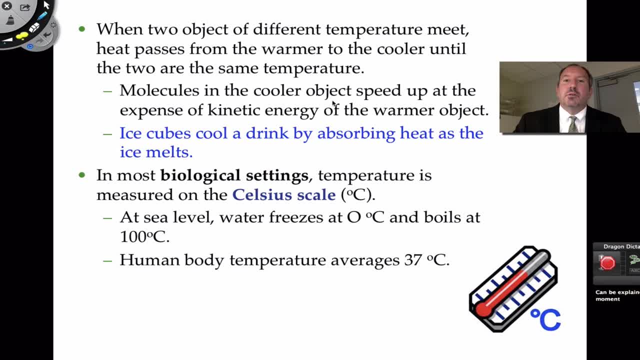 one, And so molecules in a colder object speed up at the expense of the kinetic energy of the warmer one. So in other words, ice cubes cool a drink by absorbing the heat as the ice melts. That's kind of an interesting tidbit Now. 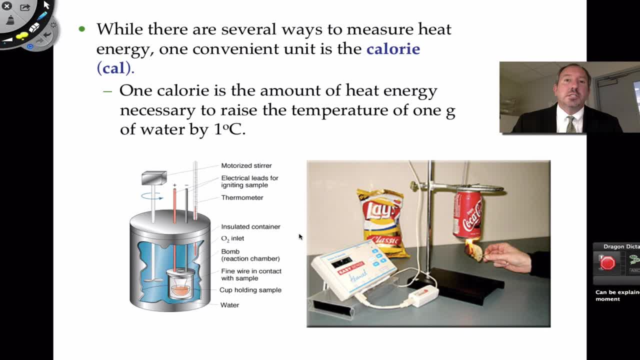 an, a property of water, or not really just water, but something that we want to consider within this discussion is the idea of calories, And so a calorie is a way that we is a conventional unit of measuring heat, And so a calorie, by definition, is the amount of heat needed to raise the temperature of the 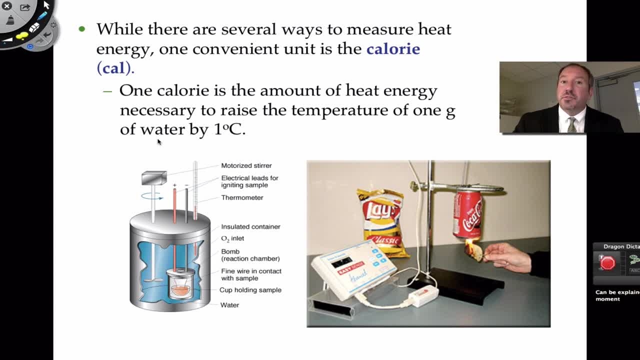 of one gram of water. so this is our standard: one degree Celsius, So one gram of water. one degree Celsius. So to determine the calories of food, for example, we can use a calorimeter that's really intense. We can put food into this chamber and we could burn it, and then it's. 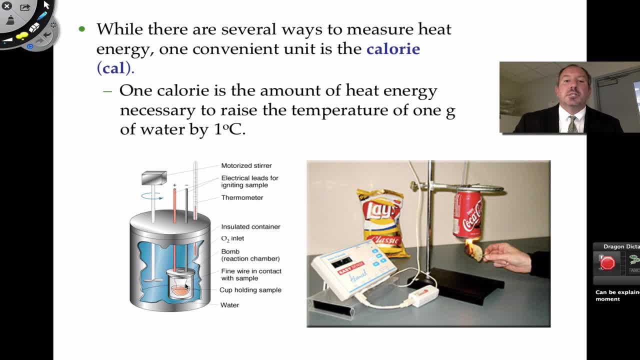 surrounded by water, and we can look at the increase and therefore determine how many calories. You might have done something like this in a chem lab. You might have taken, for example, something crude like a can and filled it up with water and then burned potato chips and see, and you have a. 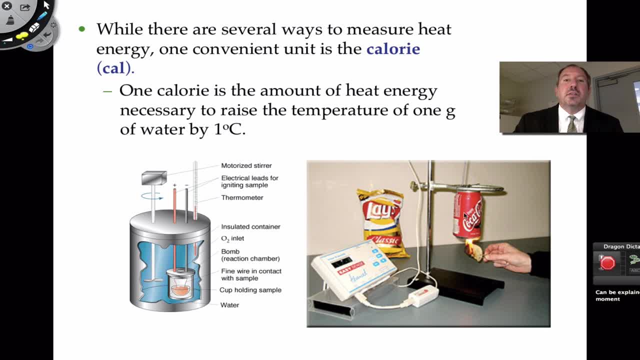 thermometer here and you try to see, or a temperature probe. you try to see the increase, to determine the amount of calories that were in a potato chip. What's interesting is this isn't best, because the heat is going all different places and it's not necessarily being absorbed. 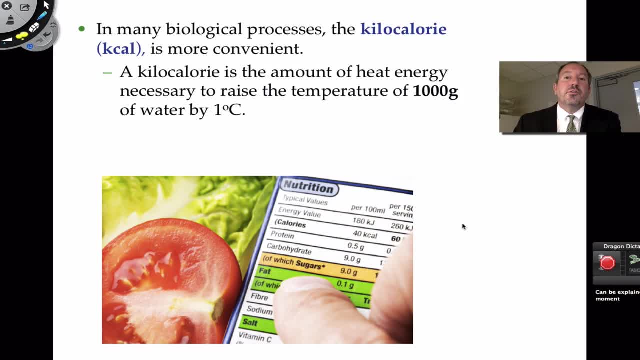 completely by the water, And so oftentimes food contains a large number of calories, and so, more appropriately, we use kilocalorie for calorie, And also a unit of energy measuring energy is a joule. This is something that we use in physics. 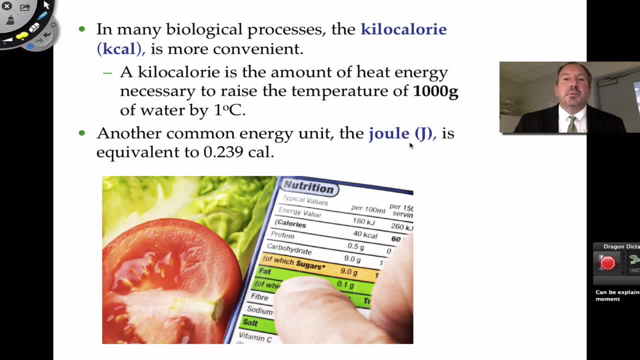 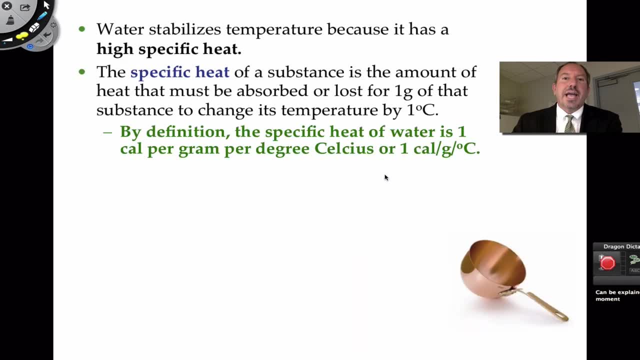 quite a lot joules of energy and this is the conversion between a joule and a calorie, if that's important in some way. So another interesting aspect of water is when you talk about specific heat. Specific heat is defined as the amount of heat that a substance absorbs or gains for one gram of that substance to 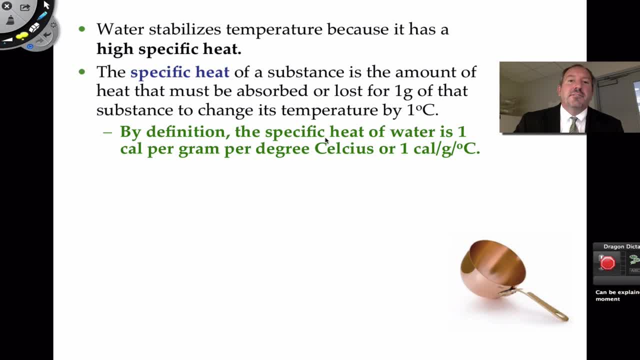 change one degree Celsius, And so the definition of the specific heat of water is one. So it's one calorie per gram per degree Celsius. So water has a specific heat of one. and you're like: why is that important, if anything? Well, what's unusual is that that's a pretty high specific heat. Now, when you compare the specific heat to other things like ethanol- 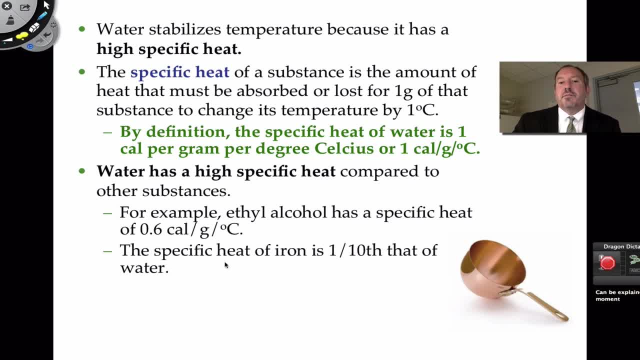 ethanol has a very low specific heat, And then you throw in things like various metals, Like we like to cook with iron, And the point of this is is that the pot gets very hot when you put a pot on a stove, and copper is even more so. 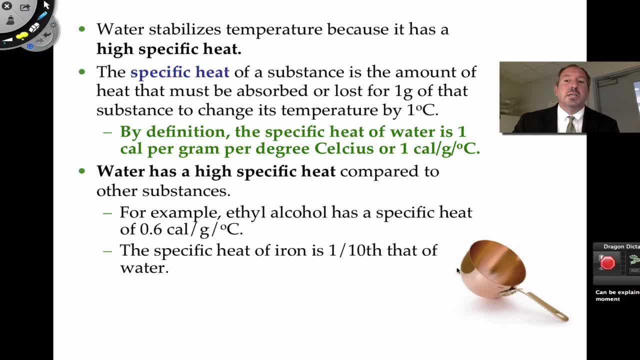 Like copper, is a great metal to use when you're cooking, because it gets hot very, very quickly, quickly, and so it's able to change temperature extremely rapidly, whereas water doesn't. so, in other words, you would never- when you're boiling water, you would never touch the outside of the pot because it's very hot. but you could. 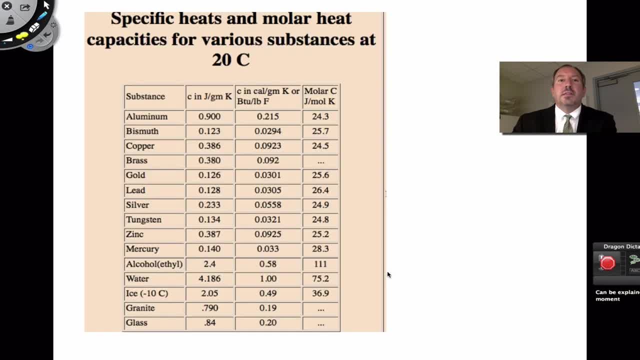 put your finger inside the water and it's only maybe lukewarm, and that's because it water has a very high specific heat, and so I thought I'd give you this chart to show you. look at, this water has a pretty high specific heat as compared to some of these other elements, and so that that's kind of 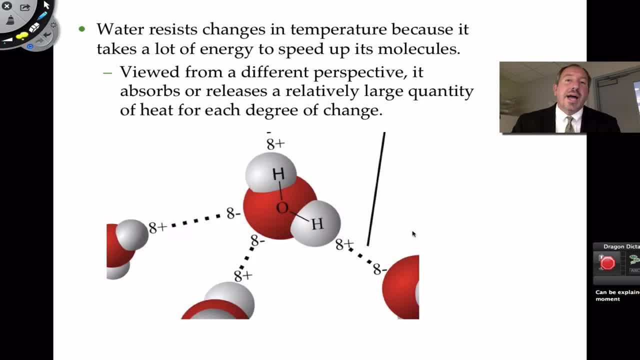 interesting, and so the reason that it has a high specific heat is- yes, you guessed it- hydrogen bonds. and so what happens is when you're boiling the water or you're applying heat to the water, it takes a lot of heat energy to break the hydrogen bonds, break the hydrogen bonds, break the. 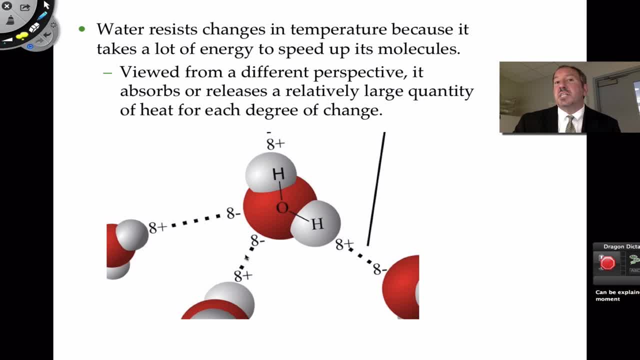 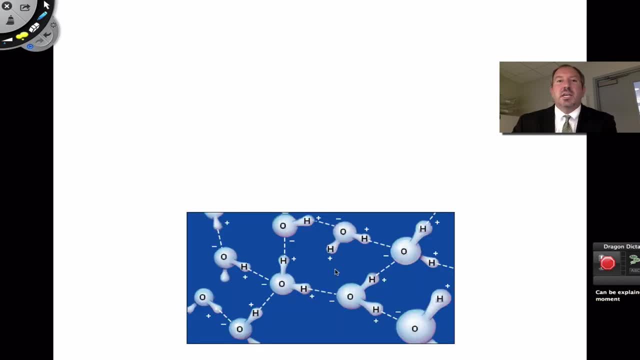 hydrogen bonds, and so the water resists changes in temperature because of the heat of the water, and so the water resists changes in temperature because it's using the heat to break the hydrogen bonds and it's not actually influencing the movement of the molecules in terms of speed, which is the 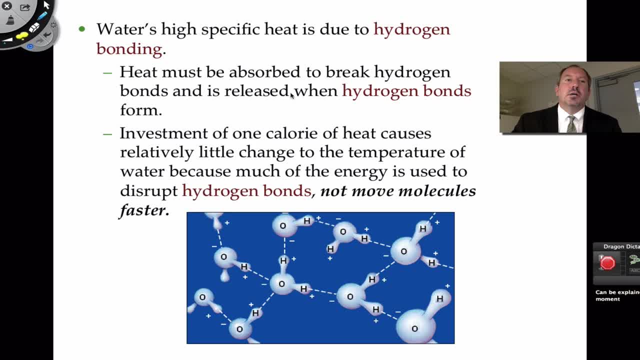 temperature is what you're considering here, and so water specific heat is due to hydrogen bonds, and so hydrogen bonds, when you break them, it requires heat to break them. so, in other words, water can really take it. it's like a sponge for heat, if you. I mean, that's it maybe a little bit off of an analogy, but I I like it personally. 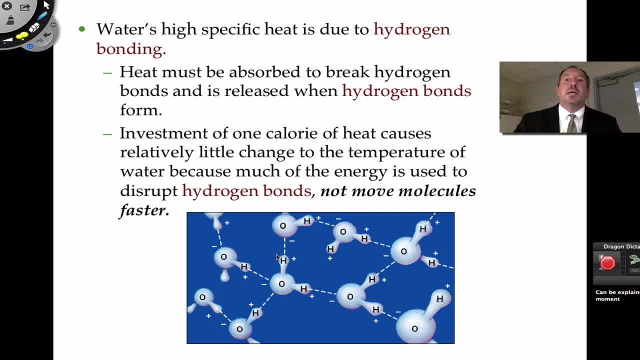 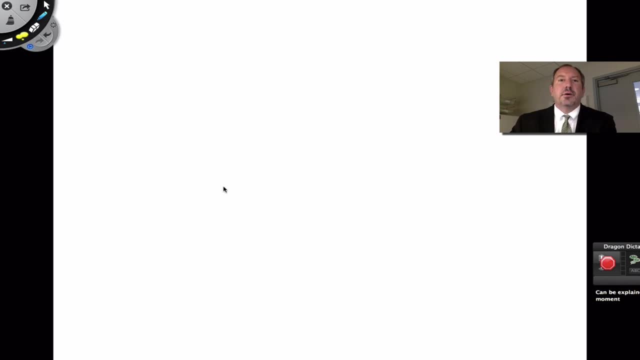 in other words, it can take it. it can take a lot of heat, take a lot of heat before it starts changing temperature, and so likewise, however, when it's cooling, then it new hydrogen bonds are forming, so it releases heat, and so that's kind of interesting and so significance. well, the high specific heat. 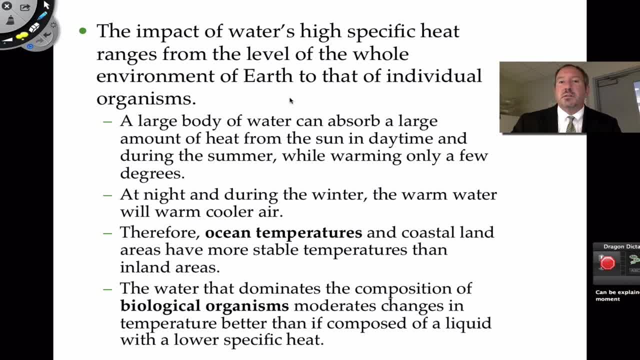 you can look at it in terms of like. you can look at it in terms of like- its impact on the earth, and you can look at it into the impact of on an. its impact on the earth and you can look at it into the impact of on an. 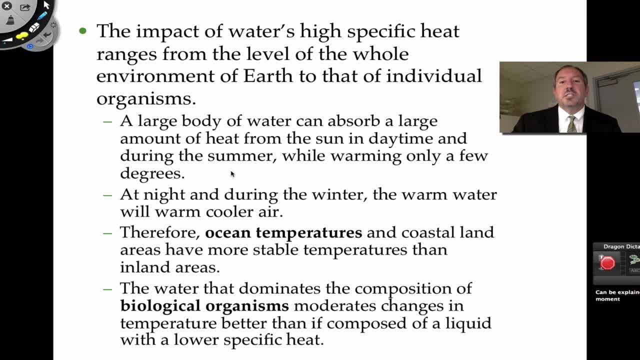 individual organism. both are important. so, like I mentioned this before, like in individual organism, both are important. so, like I mentioned this before, like in the summertime, though, if you're close to the water, the water can absorb a tremendous amount of heat, sort of like a pot on your stove, and so it doesn't get. 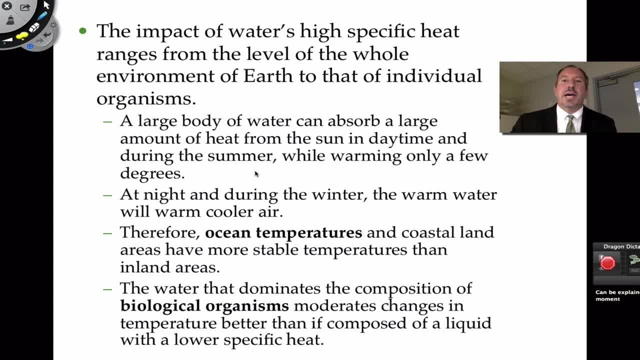 too hot, whereas if you moved inland, like for example in California, all it takes is to is to travel east, away from the Pacific Ocean for about twenty, thirty miles, forty miles, and it starts getting very, very warm. the water buffers the heat. likewise, it doesn't get very cold at night. it doesn't like inland it can. 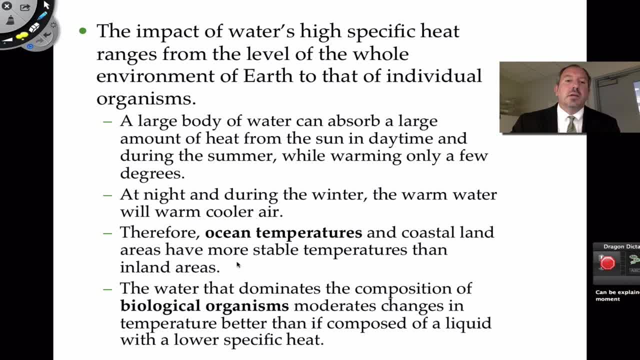 get pretty cold. but a clue on the water: it doesn't. and so in a biological organism- you want this. it's like a cooling system, like in your car. you have water circulating. in a coolant system, you have water and it helps to keep our body temperature from getting too high. in other words, it's able to absorb what. 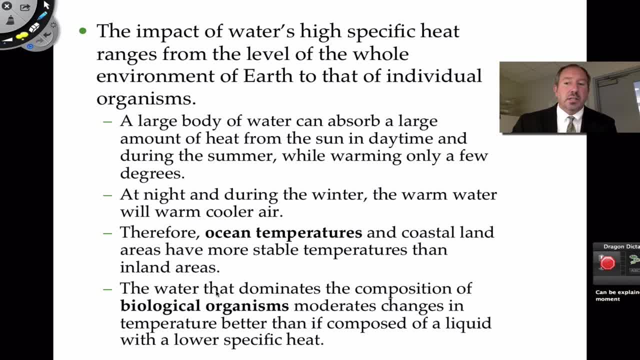 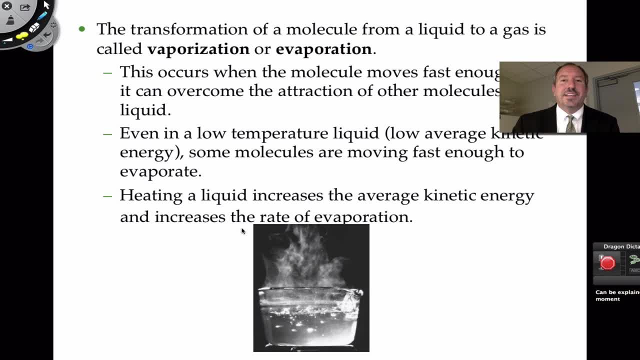 a lot of heat, because metabolic reactions often release a lot of heat, So the high specific heat of water helps us to stay alive. Basically, that's pretty important. And so here's something like when you take water up to 100 degrees Celsius and it starts to evaporate like this, you know. 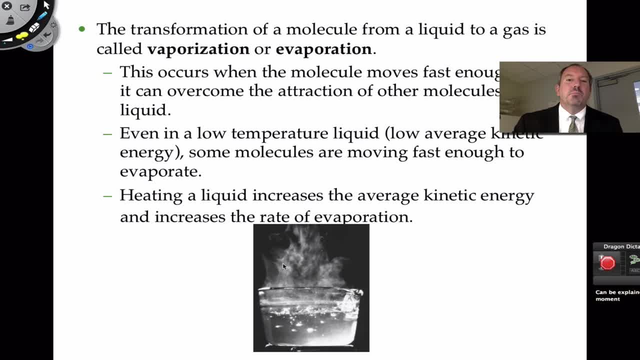 it takes a long time because of the specific heat. What we mean by this. when it starts evaporating, this is called vaporization, And so this is where the water molecules are moving so fast. Again, think of that analogy of holding hands with your friends So you're breaking. 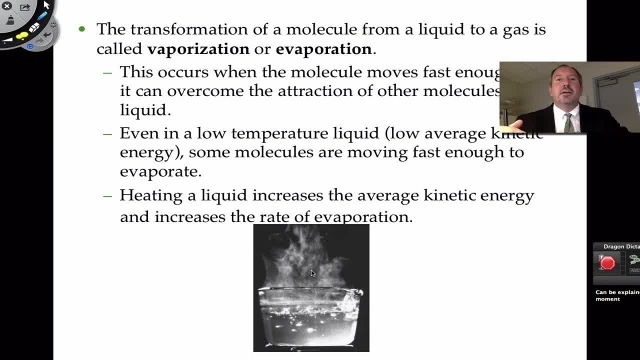 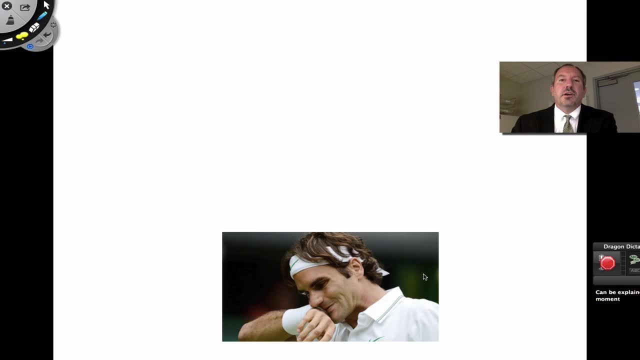 reforming, breaking, and then you take one friend and whip them right out, And so they, like, fly out of the room. So when the warmest molecules of all are the ones that are evaporating, And so the ones that are a little cooler are left behind, And so that's fairly significant when it comes to 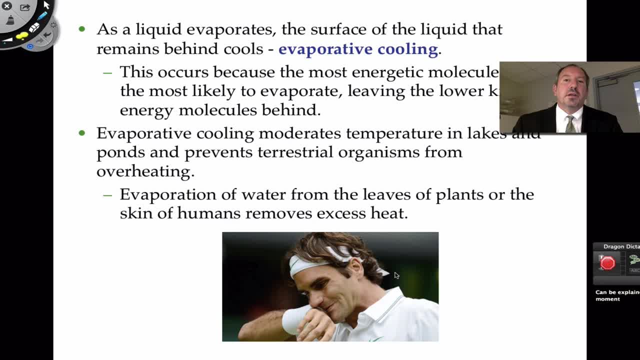 evaporative cooling, Like, for example, like if you're an athlete and you start to sweat, you know why does that cool you down? Well, as it turns out, the warmest water molecules- and this may seem weird, like I'll just do this- The warmest or fastest water molecules are the 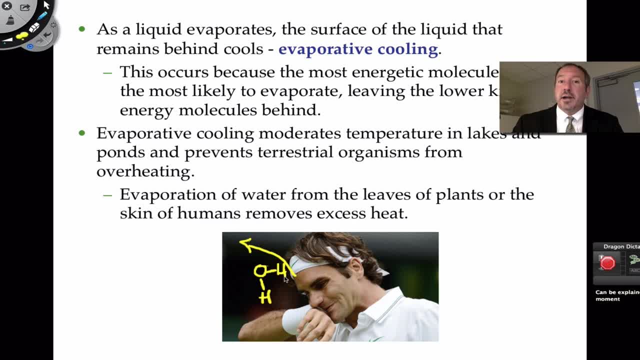 ones leaving when you perspire. Therefore, the water molecules remaining are relatively cool compared to you're like losing the fastest water molecules, And so that's that's pretty important, And so if you're ever getting out of a swimming pool, for example, 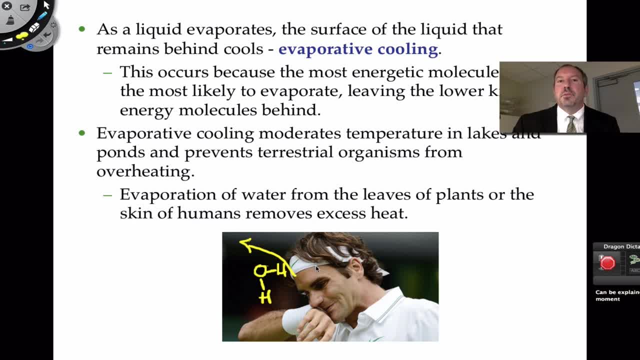 and you're cold. the idea would be to to remove as much water as you can, because the evaporation of water is what cools you. The fact that there's water on you is what's making you feel cold, because the warmest water molecules are evaporating. That makes sense. 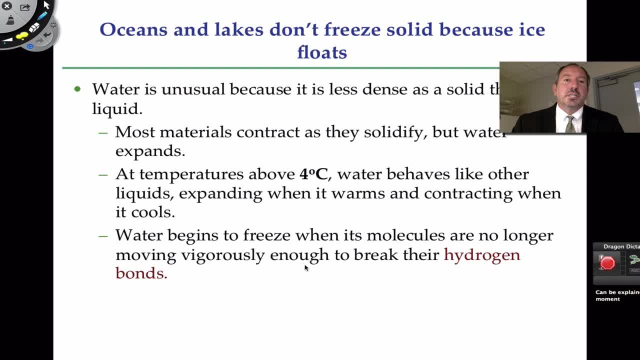 So I alluded to this point a little bit before too- in the fact that the density of water is is a fascinating thing, Like, for example- let me try to illustrate this, Let me come over here- If you had, like a big lake, a really deep lake like this, and you had, let's say that there's. 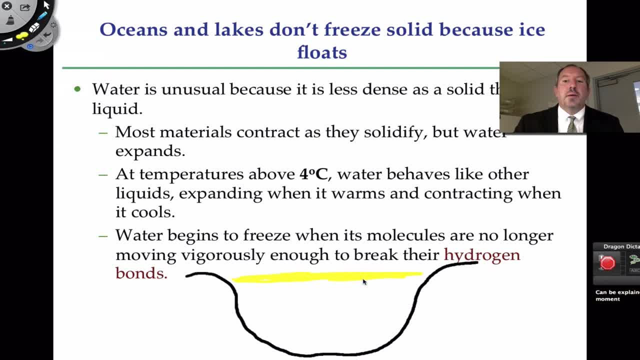 ice on the top, And so if there's ice on the top, obviously that is- you guessed it- zero degrees Celsius, And, as it turns out when you look at the water down below, it's going to be warmer as you move down. So it's going to be one. 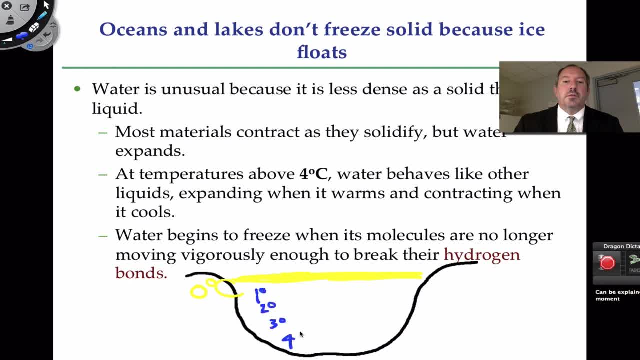 two degree, three degree- and this is kind of wild- Four degree seems to be four degrees Celsius seems to be the most dense for water. It's an interesting property, But the point being that, since water is below, it allows organisms to survive in the wintertime, They can survive. 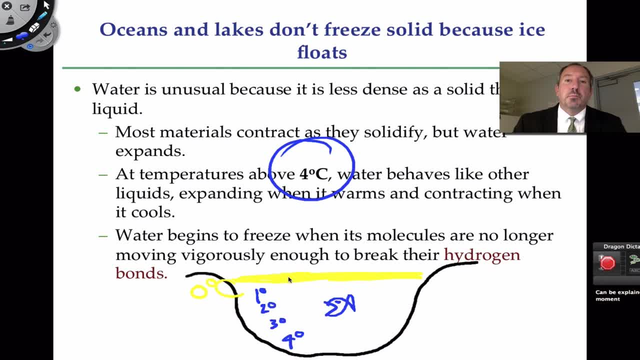 down in here. If water was, if ice was more dense than water, the whole lake would freeze over and it would devastate the lake. And so if you had a big lake and you had ice on the top, you could survive in the lake, But since ice floats, organisms are able to survive below it. 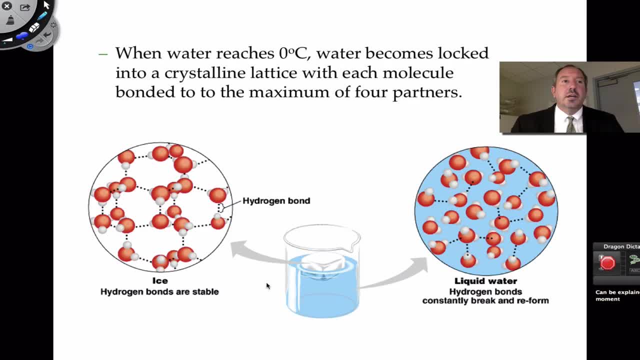 because it's a little bit warmer. And so if you ask someone on the street why does ice float? And they would say ice floats because it is less dense. But then if you follow that up and say why is frozen water less dense, I think this picture really hits it If you look at the same. 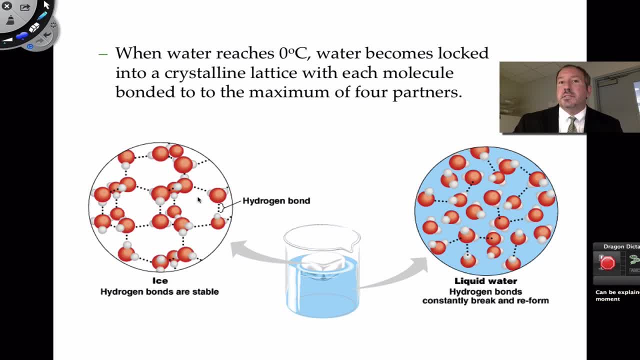 area and the number of molecules per area, which is what density is: mass over volume. you can see there's less water in ice and there's more water molecules in liquid, And that is because the molecules are moving so slowly that they can form all four partners, And so you can. 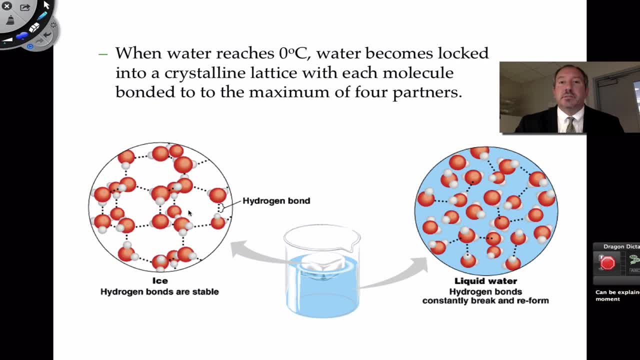 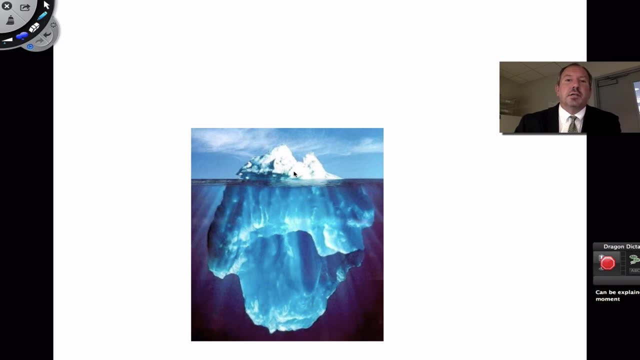 see there's a lot of space in ice less dense. These are breaking, forming, breaking forming, breaking forming, So you get more water molecules in the same area in liquid water. So therefore, ice floats. This is significant, So I thought this is kind of cool An iceberg. you may know this. that just the tip of the iceberg. 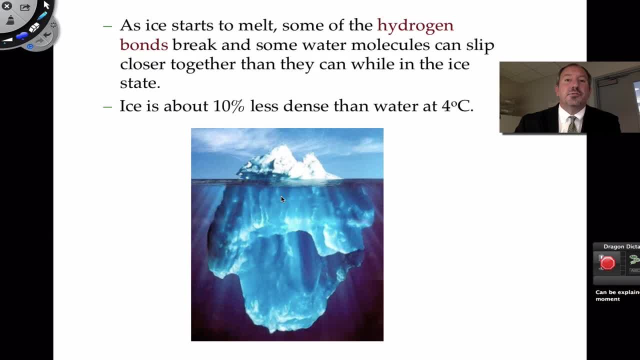 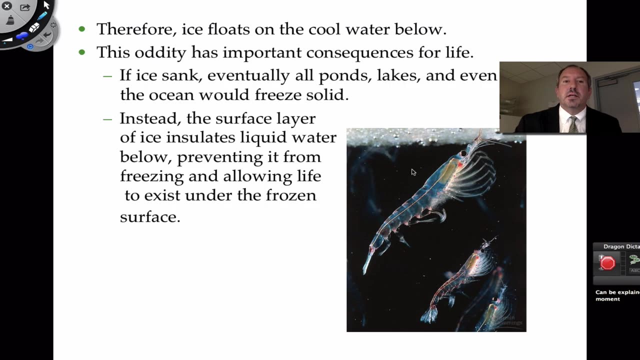 look how huge it is below. It's kind of scary. And so ice floats. it's about 10% less dense than water at four degrees, which is when it's most dense, And that has to do with hydrogen bonding. And again, this is significant because, since ice floats organisms that live in ponds. 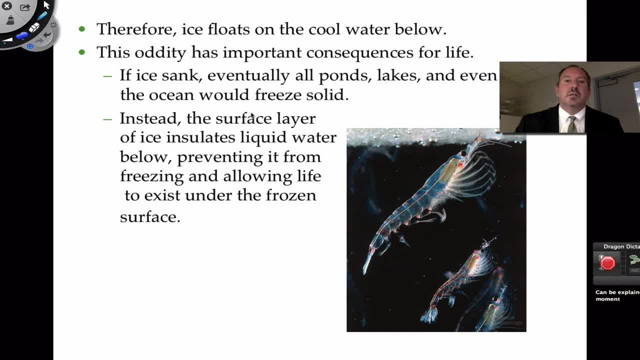 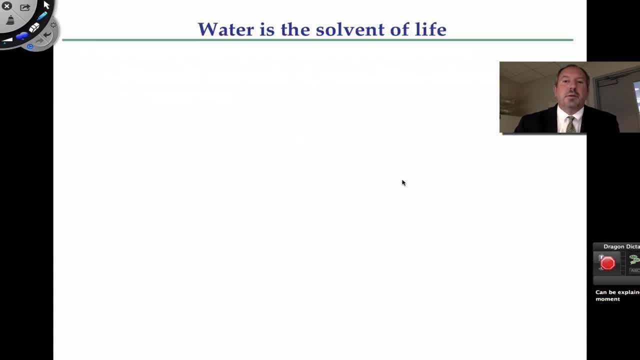 that freeze over, or a lake, even the ocean. you'd be in trouble if ice was frozen on the bottom, And so it's on the top, And so that's kind of cool, And so one of the last topics I want to discuss about water is that water is a great. 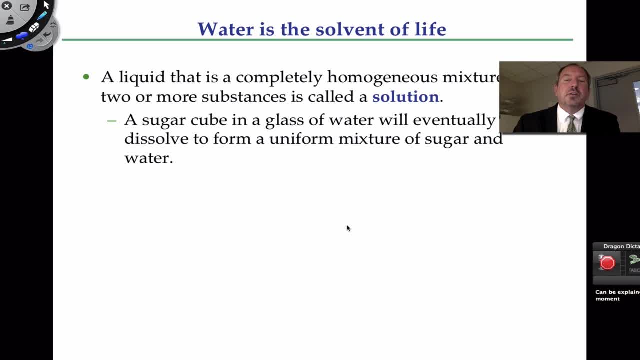 solvent. It's not the only solvent, And by being by solvent, by definition is the substance of which the solute is dissolving. And so when you mix two things together, if it's a homogeneous mixture, in other words the materials are equally distributed in the mixture, then the 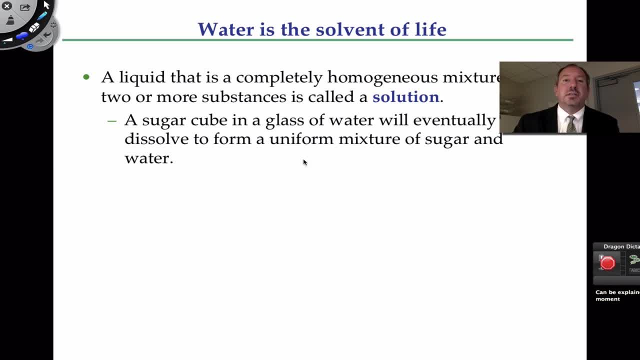 mixture is considered to be a solution. That's a chemistry definition, And so if you mix sugar into water and stir it up and it's uniform, you have a sugar solution. And so there's different kinds of sugar and the sugar would be the solute. the water dissolving agent would be the solvent. 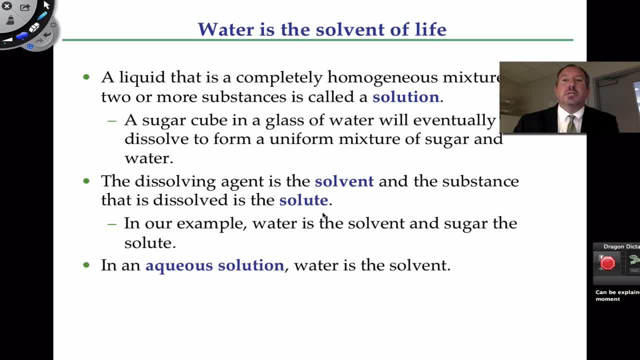 And so this is what you get. You can get a sugar solution, you can get a salt solution, And so a lot of chemicals in biology are in what we call an aqueous solution, in which water is the solvent, And so it's not the. it's not the only solvent, but it helps to dissolve polar molecules very. 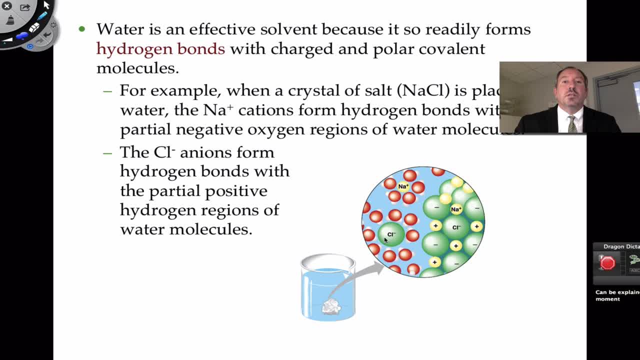 easily. Not only does it dissolve polar molecules, it really dissolves ionic bonds really well as well, Because when you put sodium chloride into water- because water is polar- it causes the ionic bond to disassociate, In other words ionize into sodium ion and chlorine ions, And so this: 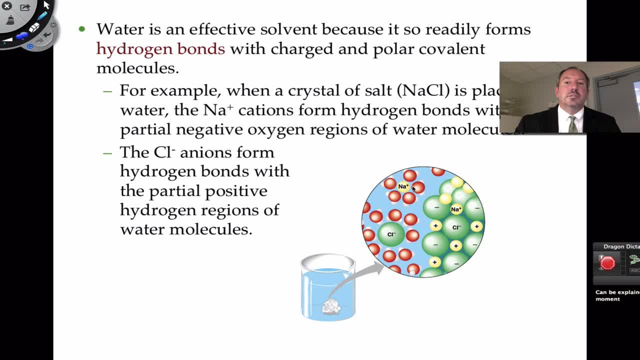 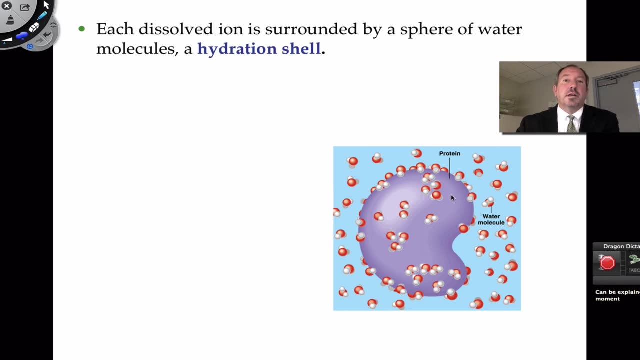 creates electrolytes in the water, And so there's a lot more sodium ions and then chlorine ions as well, So cations and anions form when you, when you dissolve salt into water. Also, you can throw protein into water. What's interesting, there is proteins, you may know contain amino acids with 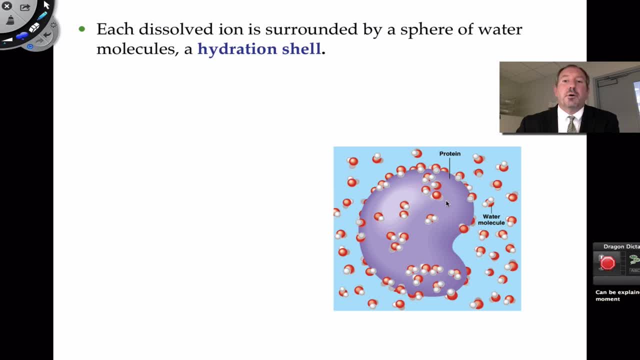 various charges. Some of them are positive, some are negative, some are polar. So what will happen is water will form like this: this hydration shell around a molecule, And they will orientate to the, to the electrical charge that's appropriate in the molecule. 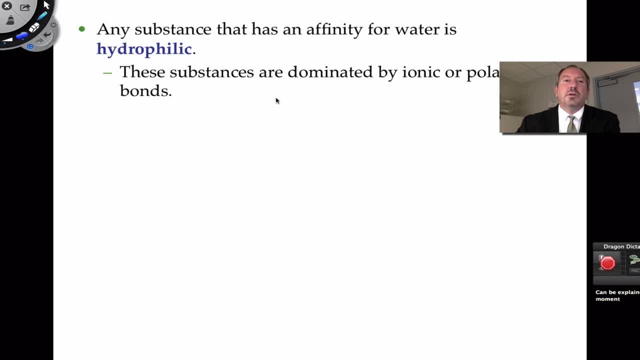 So that's kind of interesting. And then, finally, when you talk about water, it can attract to other hydrophilic molecules, Like if I drew something like this: this is not hydrophilic, These are nonpolar covalent bonds. But if I threw in this right, 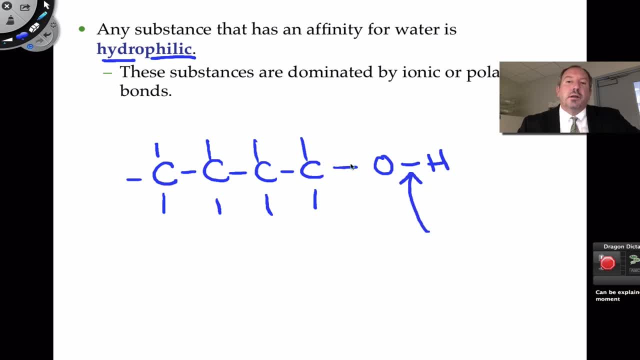 here. in other words, that, right, there is a polar covalent bond. All of these are nonpolar. Since that's polar, I can do this. I could say: this is where a hydrogen bond would form with water, And so water would be attracted to this region of the molecule, And so this area, right. 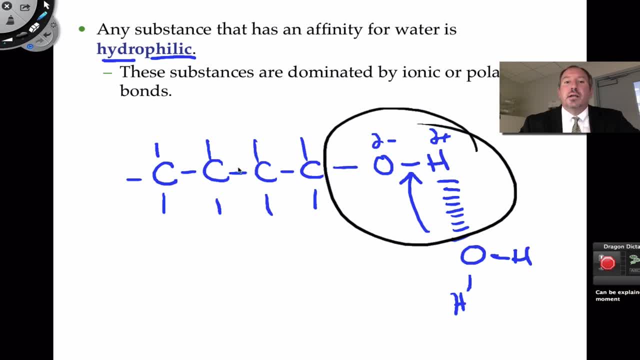 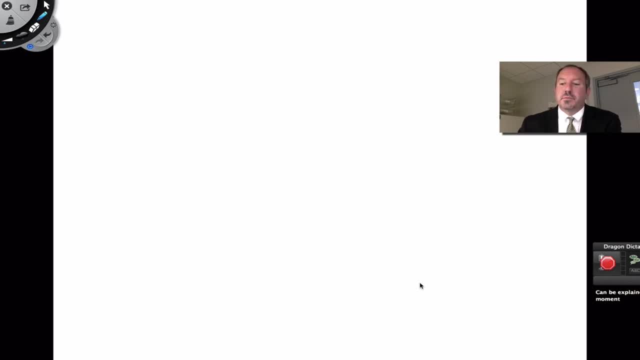 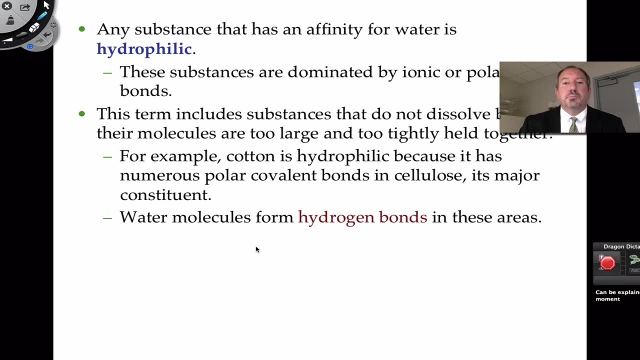 here is thought to be water loving or hydrophilic. This is water afraid over on that side And so the water. you know why? hydrogen bonds, So I went through that a little quickly. So cotton is a great example of something that has a lot of OH bonds to it and sugar in general. 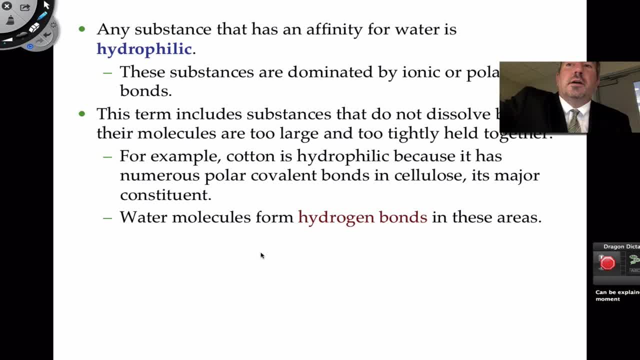 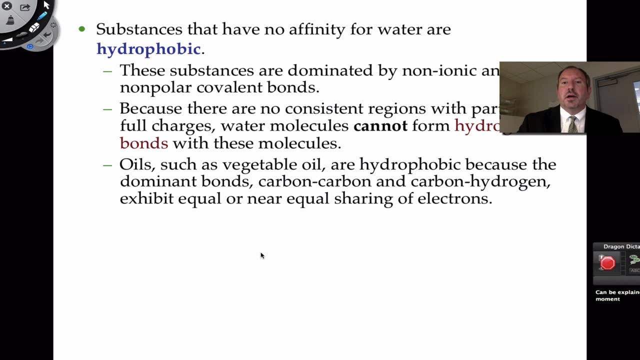 So that is why, like a paper towel, like, for example, if I took paper like this and I were to dip it in water, water would adhere to it because paper is extremely hydrophilic, As opposed to you're. like you know, I heard that oil and water don't mix And of course they do not mix. 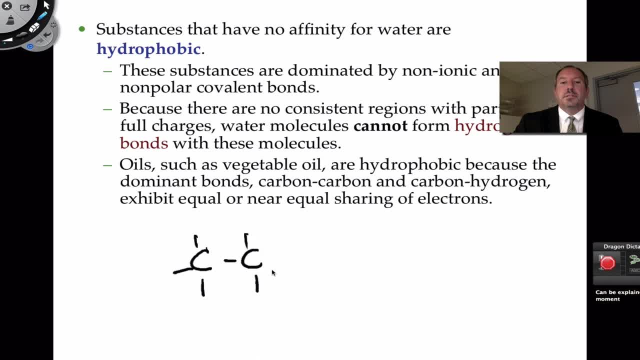 because oils are mainly hydrocarbons And there's no polar polarity, And if there's no polarity, there'll be no hydrogen bonds, And so water would not be attracted to it. So oils and waters don't mix like diesel or 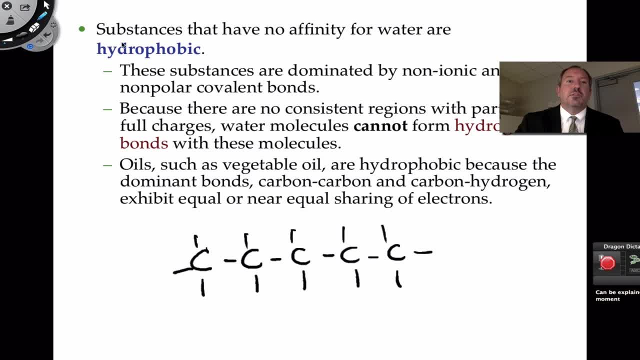 gasoline or just cooking oil, And so this is considered to be water afraid or water phobic, hydrophobic, those carbon to carbon or carbon to hydrogen bonds, And so that's important in the cell membrane. that'll come up in a different video. 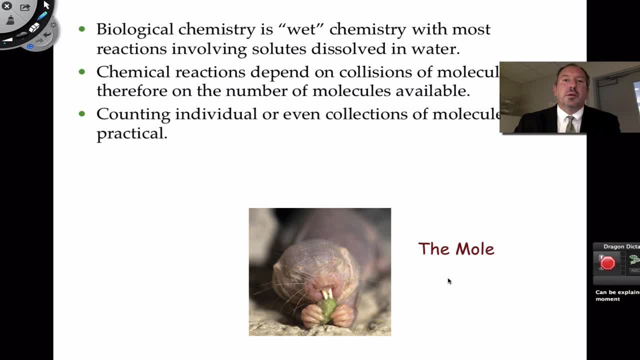 And so I mentioned that water chemistry is really crucial. So when you're creating solutions, sometimes it's appropriate, as a chemist, to use a standard methodology to determine the concentration of a solution. So we have something called molarity, which every chemist every. 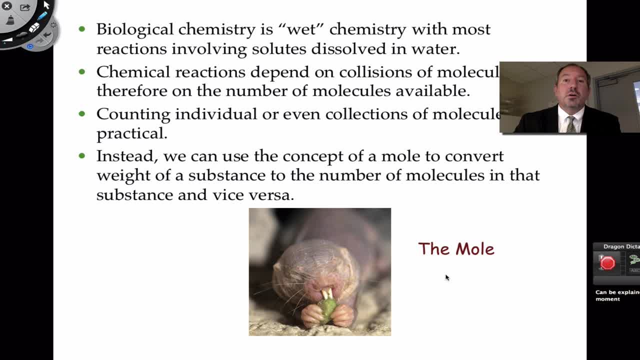 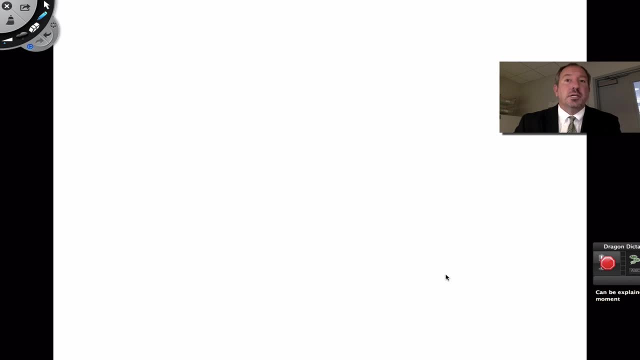 biologist understands, we use the mole concept to determine the solution concentration. because if you use a standard amount of solvent, like one liter, and you add a mole of solute, you would create what's known as a one molar solution. And the way you would do that, as a mole is the is well, you would take the gram molecular. 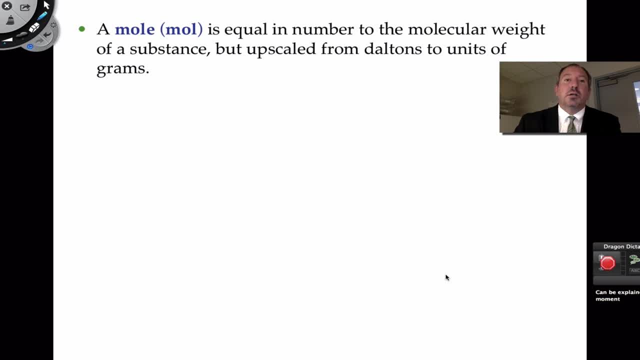 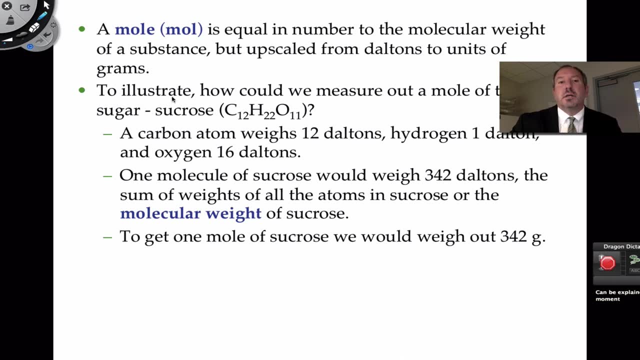 weight. Now, of course, Dalton's are very small so you can scale it up to grams. So you depends on what you're dealing with. if you're dealing with table sugar like sucrose, the gram molecular weight would you? you take the empirical formula. 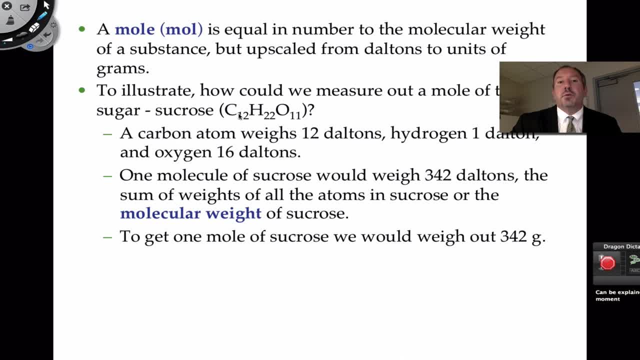 C12H22O11.. And you'd simply say: well, there's 12 carbons and the molecular weight of atomic mass of carbon is 12.. So it's 12 times 12.. Hydrogen is one, so it'd be 22.. The atomic mass of oxygen is 16.. So 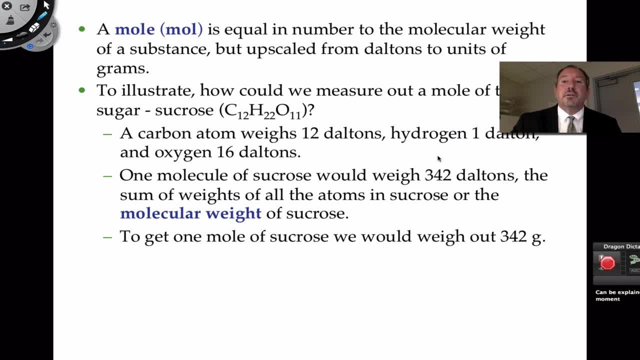 that's 16 times 11.. And you add all that together and you get 342.. So you just change that into grams. So if you took 342 grams of table sugar and put that in into a volumetric flask and then you took it up to a liter of water, 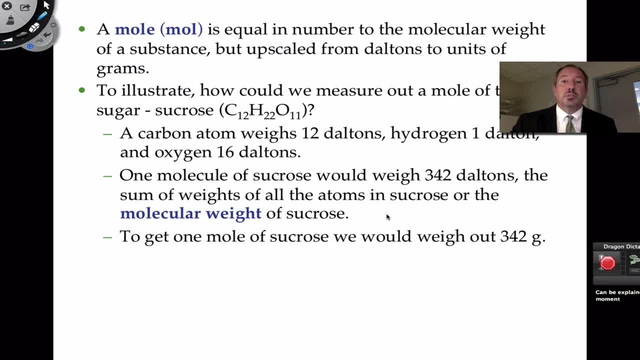 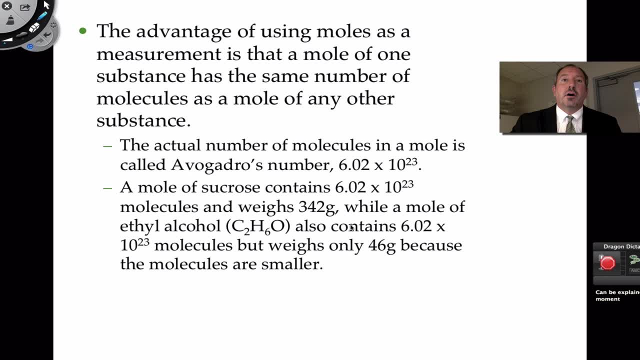 and that's the solvent. you would have created a one molar solution. Okay, and so this changes depending on what you're dealing with, Like if you have salt, NaCl or glucose, which is C6H12O6.. But